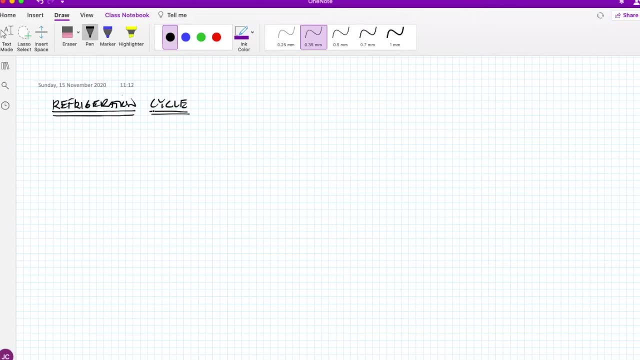 that has to do with absorption. That's called the absorption cycle, The absorption cycle. it's a little bit uncommon, So we're gonna take our lead on the compression vapor. okay, So, compression of a vapor, And you will see why this cycle has this name. Okay, so let's just see what. 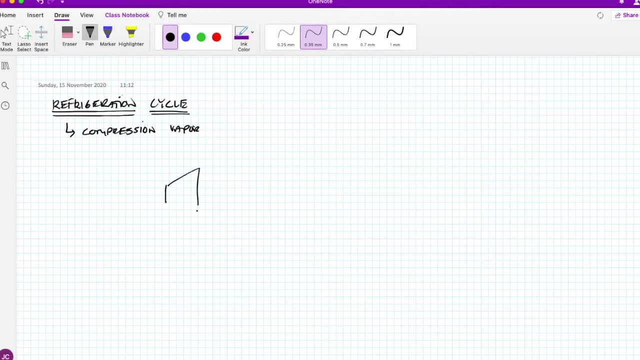 I mean by compression vapor And you need to take a compressor. okay, So there's a compressor. okay, So there's a compressor And you need to take a compressor. okay, So, there's a compressor here. It goes in here at one And then it goes out at two, Yeah, And then comes to a heat exchanger. 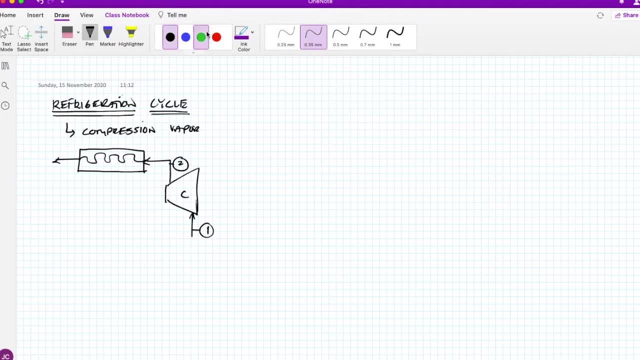 This heat exchanger provides the outlet of heat, So I'm gonna put QH. H is because of high, So what I mean by this is that the heat is going from this condenser into a high temperature reservoir, Which most of the time is the environment. okay, So at the back of your refrigerator you will find 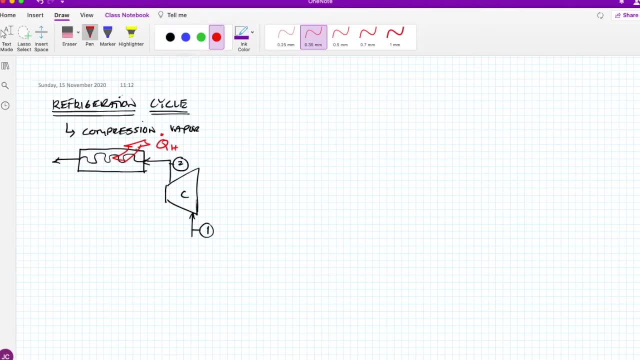 maybe some piping. There's a piping that goes around, that's snaked around at the back of the refrigerator And that thing will feel warm. okay, So that warm that you're feeling over there has to do with this heat being released by the machine. Okay, so that was is a QH. I need to tell you that. 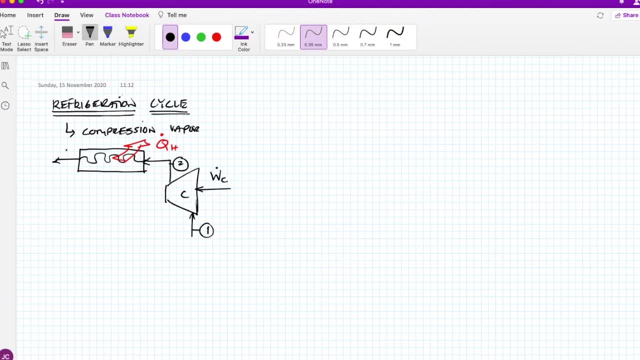 the compressor receives a lot of heat And it's a lot of heat And it's a lot of heat And it's a lot of compressor's work for the compressor. So so far you have two machines: compressor and a heat exchanger. The name is condenser In this case, this thing is condenser because there's the 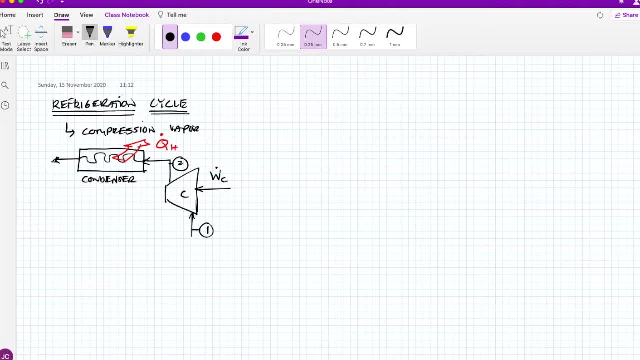 condensation of the refrigerant going inside this cycle. then you will find out about a bulb. Okay, so here at the entrance of the valve, it's a point three, and at the outlet of the volt, of course, it's point four. Okay, So these things evolved. 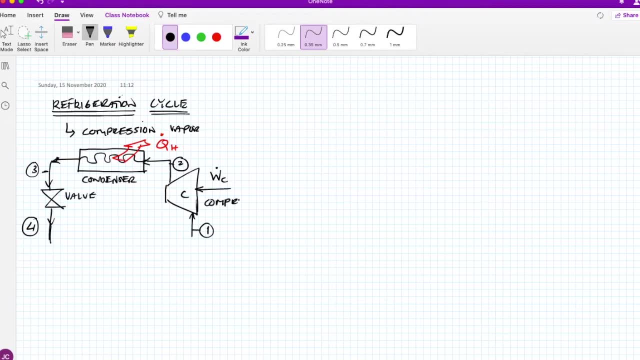 here the bulb. okay, if you want more hints, this one is a compressor and then you will find another. just to complete the circuit, you will find another heat exchanger, which is called the evaporator. the evaporator, where the refrigerant will evaporate. okay, so you have completed the circuit. inside you will use a substance called refrigerant 134a. 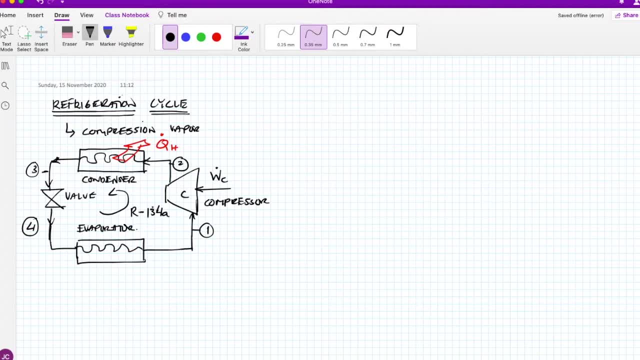 okay, that's the name of it. this is the way the refrigerants are named. it has to do with the amount of hydrogens and flours and carbons that has the molecule, because these are complex molecules. okay, so these are complex compounds and therefore they are named like this, because 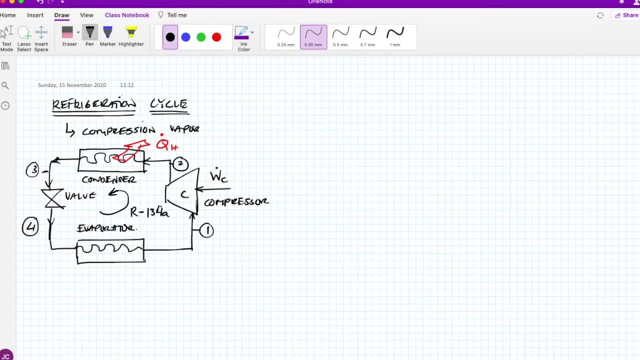 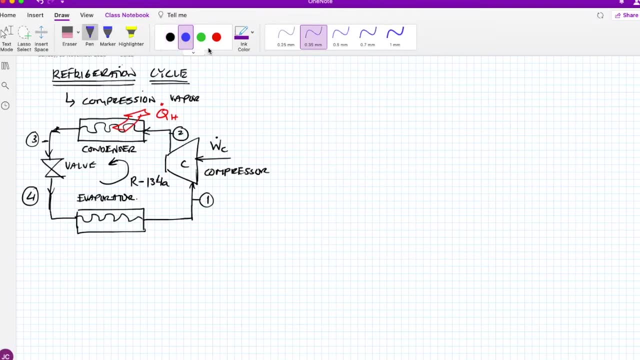 otherwise the the names are kind of long names, okay, so it's better to remember with this symbology. okay, so, here at the evaporator, you will take heat from your food. that's the whole purpose of the refrigerator: to steal heat from anything that you're putting inside the box, which is a 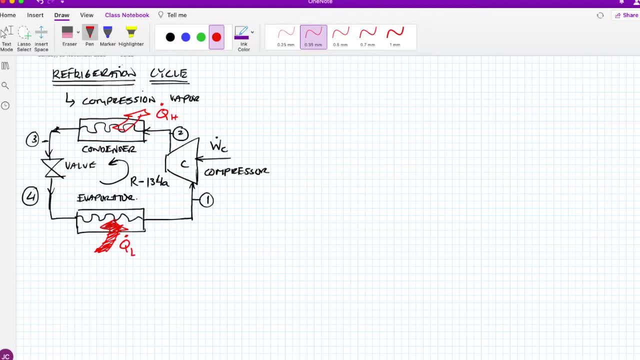 refrigerator. okay, you are putting, you are taking them heat out, okay, so those things will remain cold, okay, and there won't be any growth of bacteria that can damage. well, there's gonna be growth of bacteria, okay, but maybe it will last a week instead of just one, or 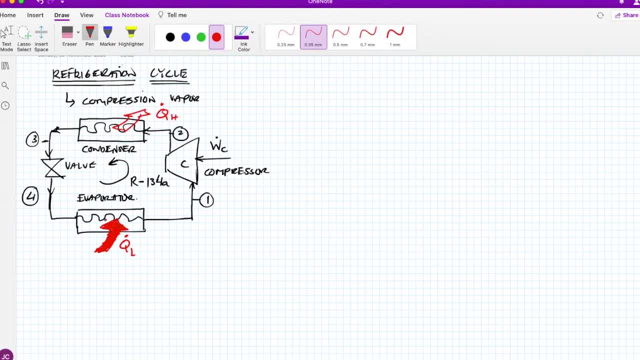 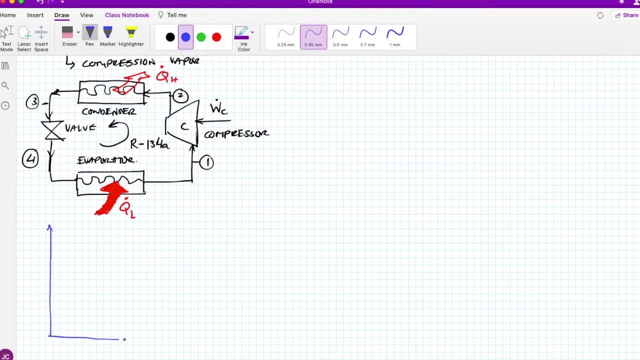 two days if you put it outside of the refrigerator. that's the whole idea of a refrigerator at home. okay, well, okay. so you have that and you have here the cycle. now let me just try to illustrate this with a diagram so you may understand what is happening here before going into the 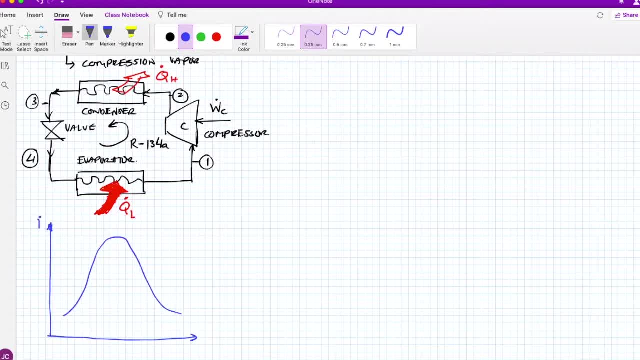 into the problem. okay, so you will have. let me just put here the pressure and this one. let me just put this one. what should i put? okay, enthalpy, why? why did i doubt or why did i hesitate about putting this axis, pressure and enthalpy? well, basically, because you can put anything you want, okay. 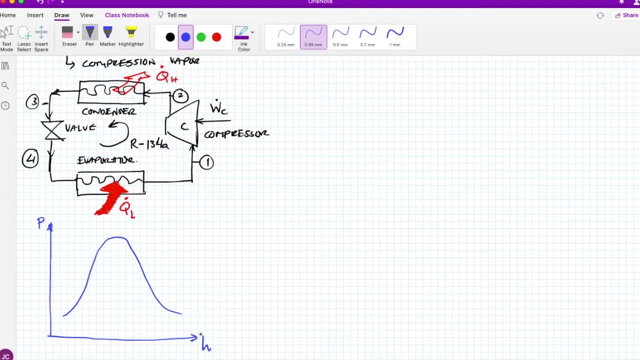 in the sense of properties. you can put pressure, enthalpy, pressure entropy, temperature entropy or something. most of the times, this is the one that you use to put the pressure and enthalpy into the in order to illustrate what is happening. okay, so i'm going to talk about the ideal. ideal. 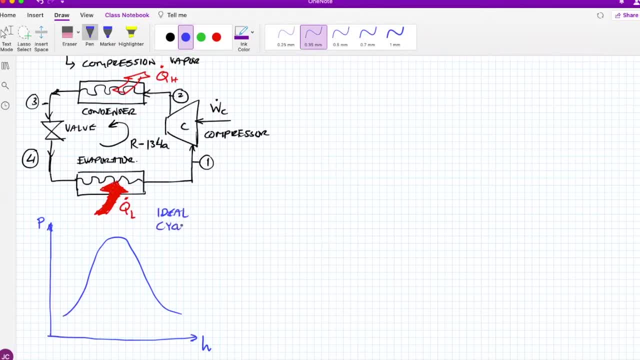 refrigeration, compression vapor cycle. so i'm just going to summarize by saying the ideal cycle, because if you got yourself with a real cycle, you will see some differences. okay, differences that has to do with maybe the machines are a little bit imperfect, okay so, but now in this one i will start. 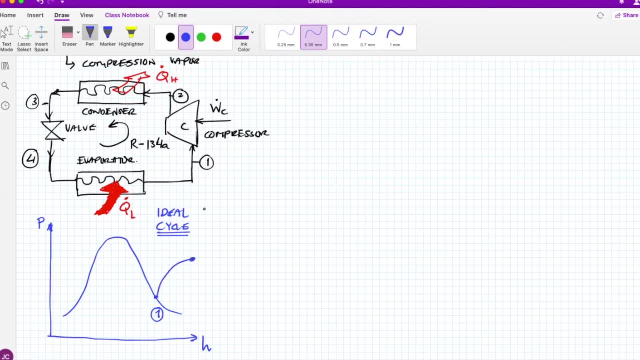 here this saturated steam, and i'm going to show you how to do it. okay, i'm going to show you how to do it, then i will compress it. so you see that this one would be two. okay, most of the time, if it's an ideal cycle, this guy means that the entropy remains the same inside the compressor. then you go yourself to. 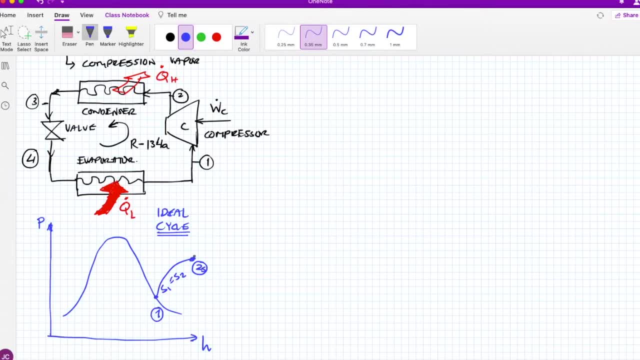 2s. let me just emphasize that this 2s is the isentropic state out of the compressor. then you will place this inside a heat exchanger, and heat exchangers tend to be okay, so i'm going to put the 2s on here. so, since we have the, the heat exchanger, we can actually cried out x2 in the. 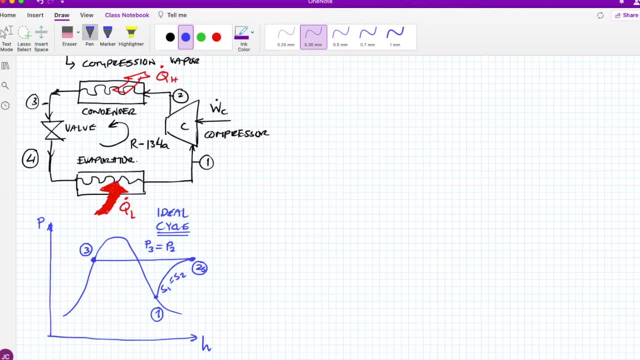 substrate, and this is one that would be the ios of tritium. okay, if you just take this one and you put this on a separate liquid, okay, and what you're going to see here is this: here is a two, okay, and you can see this: here is a three. okay, so three equals to p two- okay, so this one is gonna be. 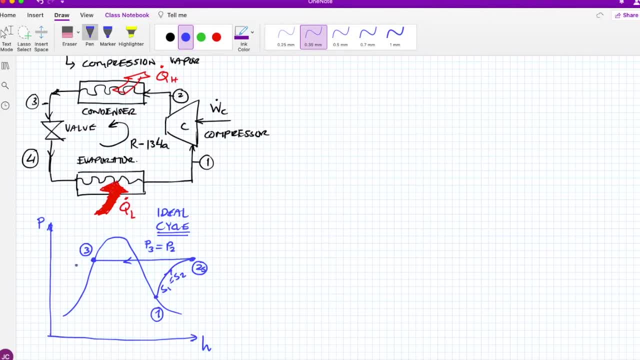 three is located right here at saturated liquid, and the process between two and three? okay, it's, it goes into a valve and what it does? okay, it does this. so it depressurize, it takes out the pressure, it reduces the pressure from three to four and it does it at the same enthalpy. that's why i have a. 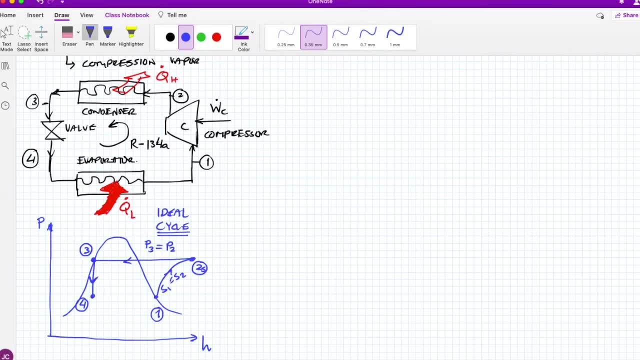 vertical line from three to four, because the process is isenthalpic. okay, how do you know this? well, that's how most of these valves work. it doesn't mean that they necessarily do it all the time in reality. but, um, but you can model it like this: now let's go for four to one in the heat. 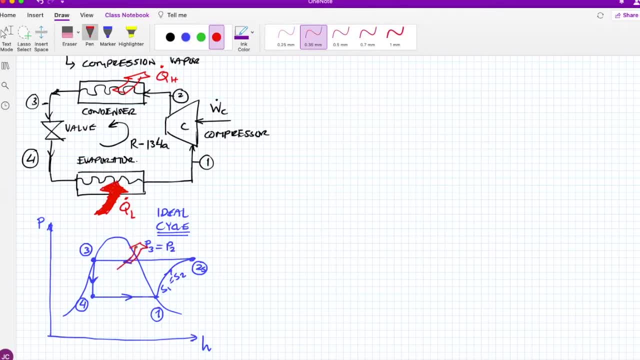 exchanger. so again, let me just try to. you already know this drill. okay, so here is a heat qh, here is the ql going into the cycle, going out of the food but going into the cycle or the refrigerant. okay, so this one is qh and this one is. 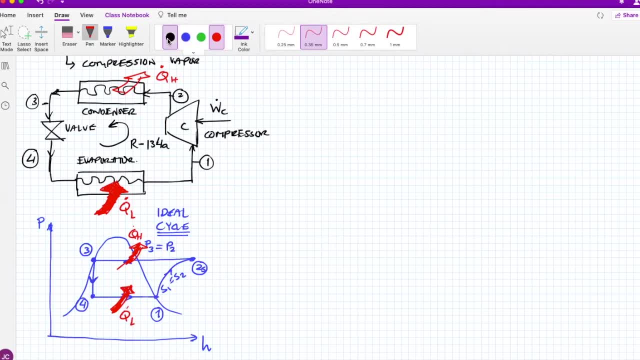 qh and this one is, and this one over here, let me just put it with, so you will have here the input of work, okay, okay, so we're going to solve a problem. let's just see example, let's just do example and within this example, i will tell you something about the indicators of this, of this, uh, refrigeration. 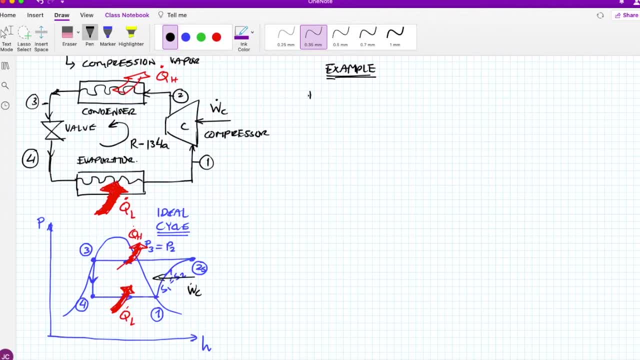 cycle. okay. so the example says like this: let's just put data. okay, let me just put the data of this stuff and which would be the temperature from the evaporator: it's minus 20 degrees celsius. okay, so that's what it is. the temperature of the condenser, of the condenser is: 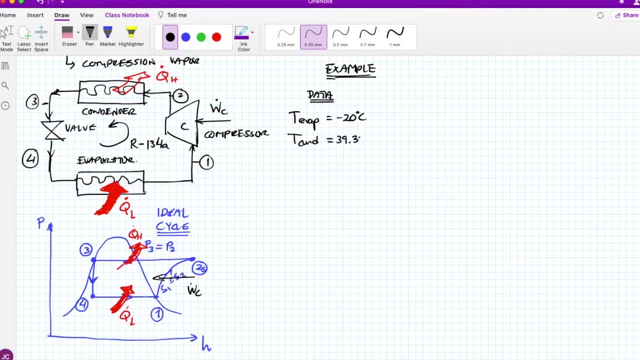 39.37 degrees celsius. yeah, i think i'm right. and the mass flow, mass flow rate, is 0.6 kilograms per second. there's not a lot of refrigerant going inside your refrigerator. okay, um so fine. it says: find a um ql. so ql is a heat power that you are. 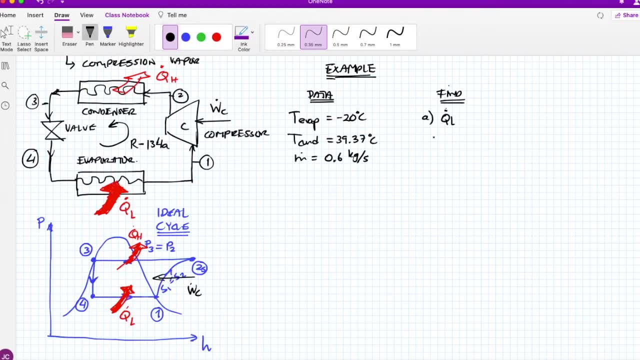 taking from the food. this is actually the refrigeration rate. okay, this is actually the. you could say that is one of the most important things, otherwise why would you buy a refrigerator now? b- uh, you need to get the cup. okay, so you're gonna get the cup and c cup. i will talk about what the 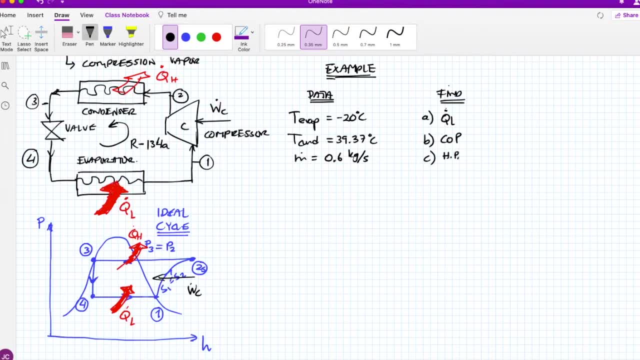 hell is. the cup c is an indicator of how much work going into the compressor you need in order to produce a ton of refrigeration. ton of refrigeration, okay. so this is a little bit weird. this is just language bite. the refrigerator would work okay as a heat pump and i will try to explain you the difference. 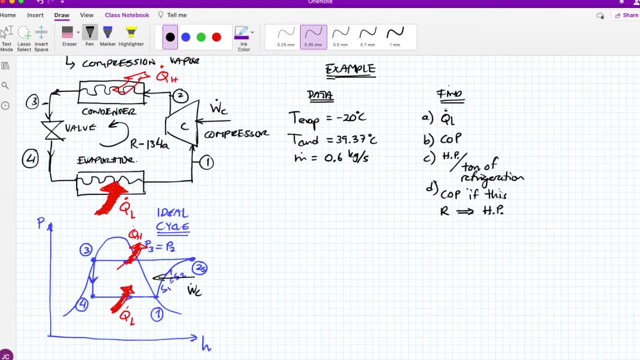 a little bit in this, in this one, okay, but you should go to your textbooks and see what is the difference between a refrigerator or a heat pump, okay. so in this case i mean by a heat pump. do not get confused with this, which is horsepower. sorry, i didn't make up this nomenclature or these symbols. 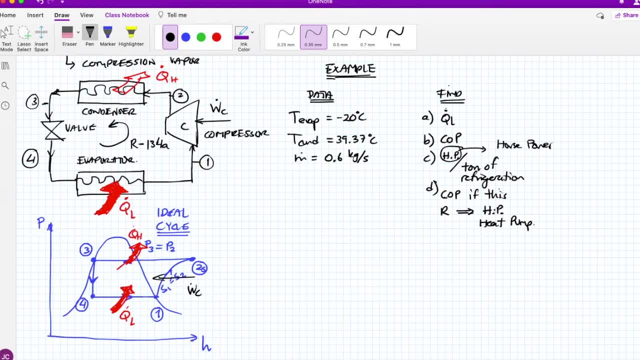 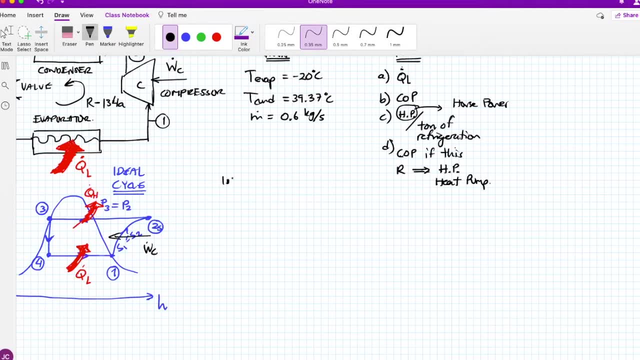 but this hp and this hp are different. okay, now let's just go and do the problem. um, okay, so the ideal cycle. let's just put here the ideal cycle. a yield cycle means that i'm gonna need some data, right? oh, my god, you're so, you're a genius, yeah, i know so. one one. 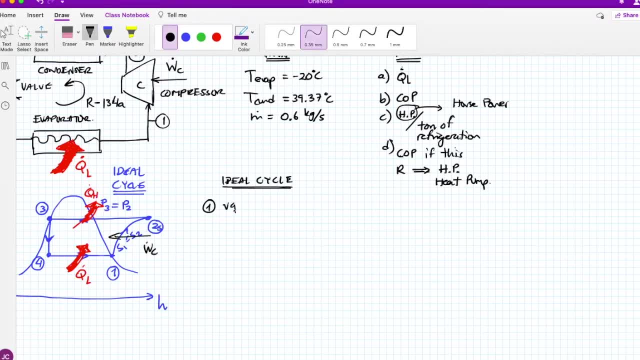 one. let's just see how i can find one. it's, um, oh just saturated, saturated saturated steam, because you are located right here at the line of the saturation curve. so saturated steam and you have the temperature. you don't know it, but you have it because it's the temperature of. 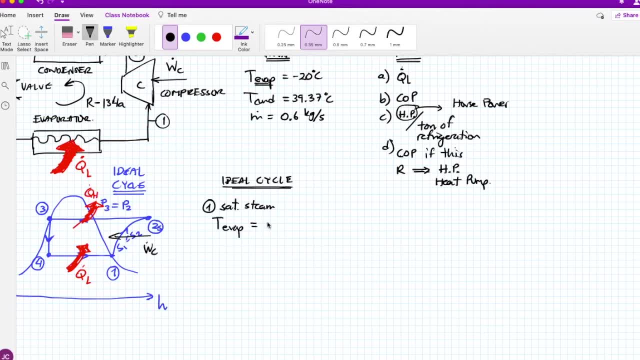 the evaporator, so the temperature of the evaporator is actually minus 20 degrees celsius. if you go to your r134a tables- okay, you can go here and find out how much so h1 would be h g at minus 20 degrees celsius and you will find yourself that h1 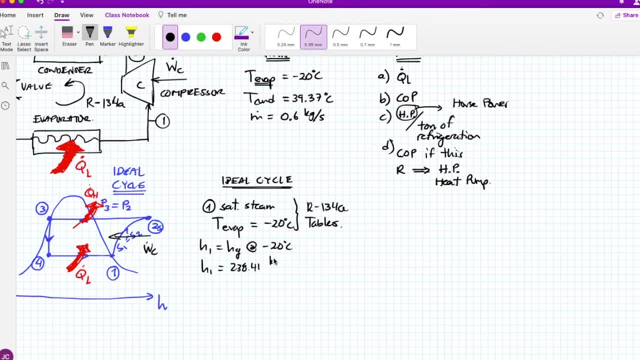 equals to 238.41 kilojoules kilogram, and also you need to find this guy. i will tell you why in a little bit, but this is the entropy at those same conditions, which is 0.94, 5 and 64 kilojoules kilogram kelvin. okay, so you have find everything you need about one. let's just 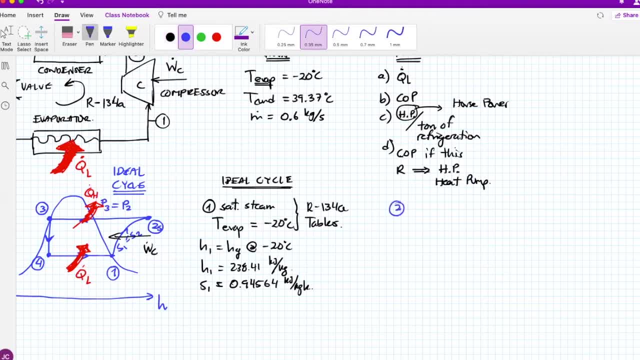 just go with two, so i'm going to put here two. so for two, you are here. it seems that you are in superheated steam. right, it seems that you're here, so let me just see what do i have. look guys, i don't have too much, at least here. i don't know what the hell i am. i think i for one, i have the temperature. 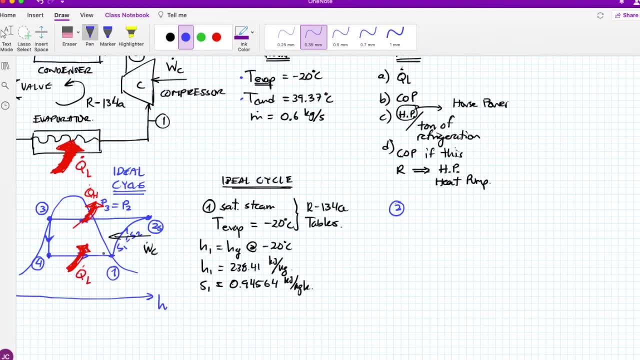 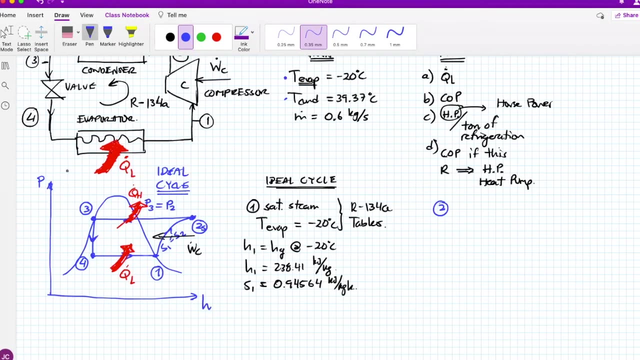 of the evaporator because it doesn't change. how do you know that? well, because i can go to my textbook. i'll read a little bit about the theory of this ideal cycle for refrigeration and you will find out that the temperature of the evaporator here doesn't change because it sticks here. okay, 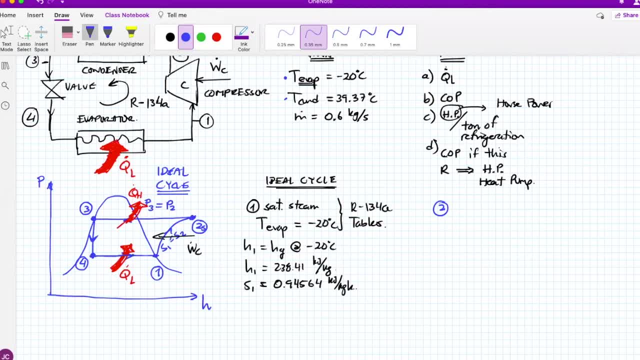 at four. then it passes. it gains heat, but not temperature. so the temperature is the same one here, inside the saturation curve, because it happens to be at the same pressure. so if the pressure doesn't change and you are inside the saturation curve, the temperature shouldn't change, okay? so that's how i know that this temperature evaporator 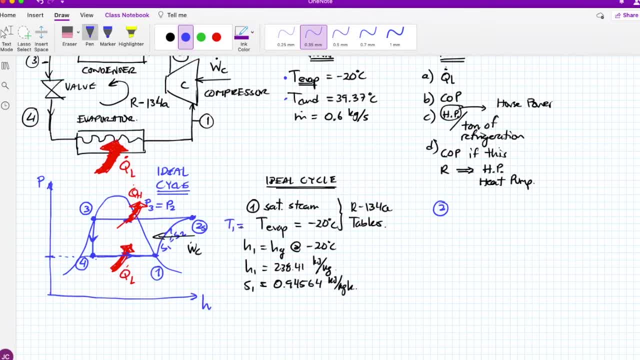 whether it's t1, this is. i can say this: t1 equals to t4. i actually can say this: that is the evaporation temperature. okay, so now at 2. i know that, oh my god, i know that s1 equals to s2. yes, i. 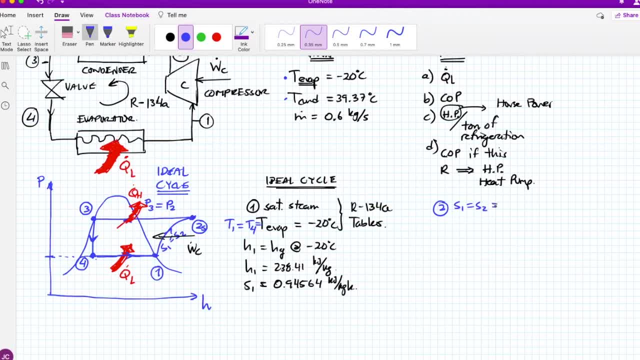 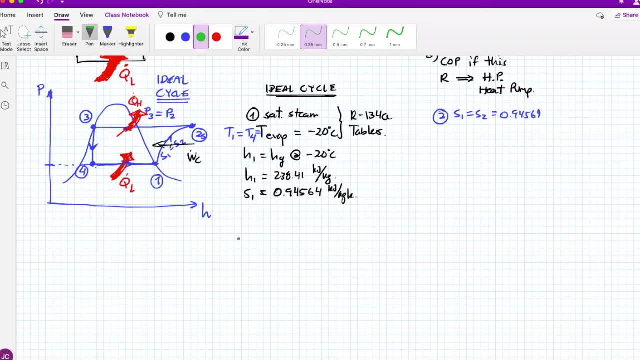 know that because it's the ideal cycle. therefore, uh, so i know this 0.94564, but i don't have anything else to work with, so it seems like you are a little bit uh, lost, right? well, let me just go here and say: okay, now let's just go to three. let me just go to three. hey, what happened to two? 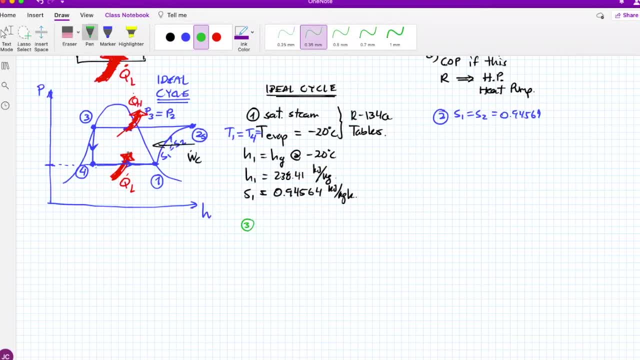 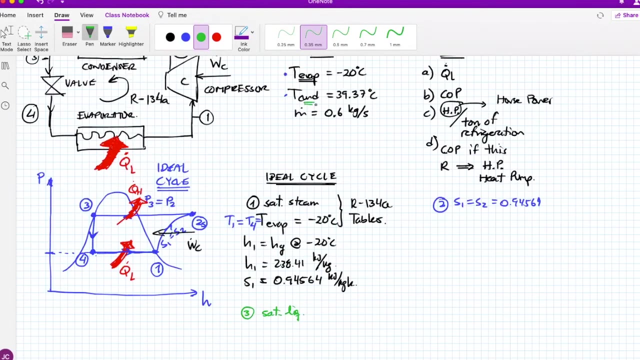 i'm gonna do it later, hopefully i can take you there. so for three, you know you have saturated liquid, okay. so you have saturated liquid and you also have, oh, okay. so now you need to start using your other data, which is now temperature of the condenser. 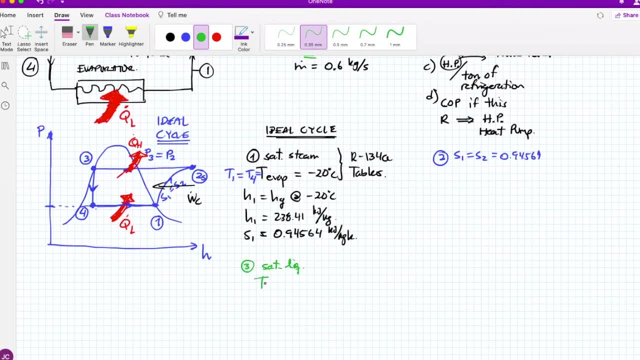 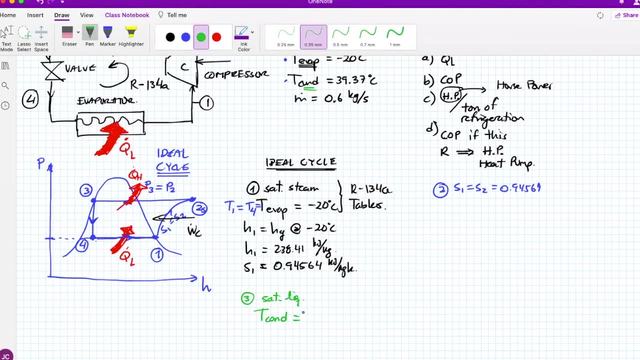 okay. so temperature of the condenser: this is not a very good established data. temperature of the condenser is 39.37 degrees celsius. okay, so i think this is, um, well, it's not a mistake part of the example, but it's something hidden here, because, look guys, the condenser is between three and two right here. 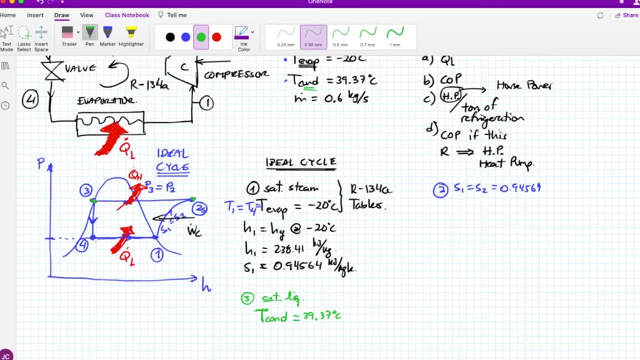 lies the condenser, and i saying i'm assuming that the at the outlet of the condenser. you will have the temperature of the condenser as my data. but you could also argue: hey, buddy, why didn't you use two? okay here, why not temperature of the condenser, of the condenser here? okay, why not use this one? 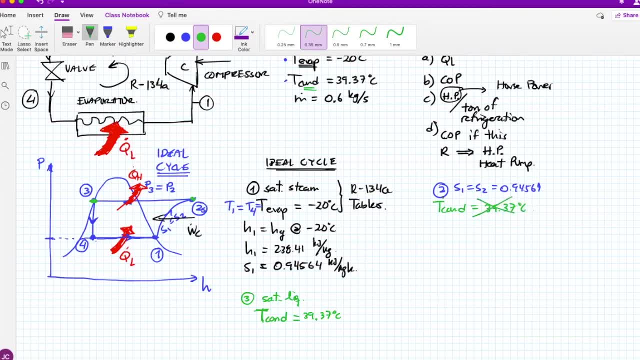 and if you do that, you would be wrong, and- and yeah, that's the problem with this type of data: they are not telling you the whole story, so you cannot use this one. maybe because of this, here you are at a superheated steam, so this temperature t2 won't be the same one as this one, because if you 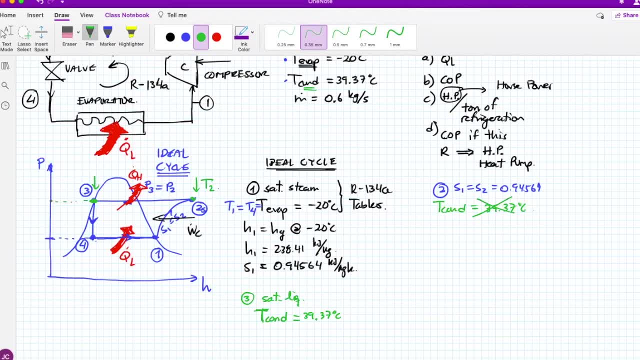 are in superheated. okay, at the same pressure. you have the same pressure. i don't know if you see this, but p3 equals to p2. that was established first. let's say we assigned at 2 degrees celsius or 1 degree celsius. it Sunday before and calendars a 2. you can find another Friedman. Oh, that's actually often. ignore that one. okay, because the total temperature is 285 degrees Celsius. 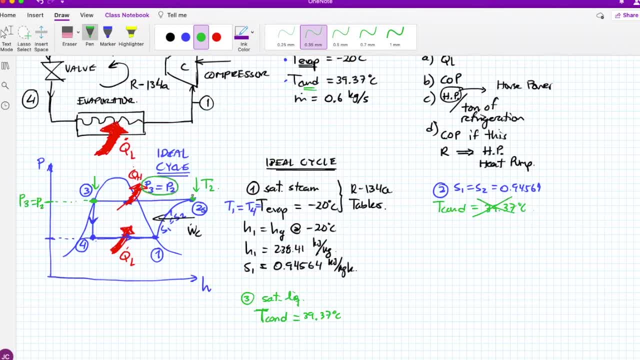 that was established already here. So P3 equals to P2, right, But the temperature is not the same one because you are not inside of the saturation curve, as you were here from four to one. okay, From four to one, you were inside the saturation curve. 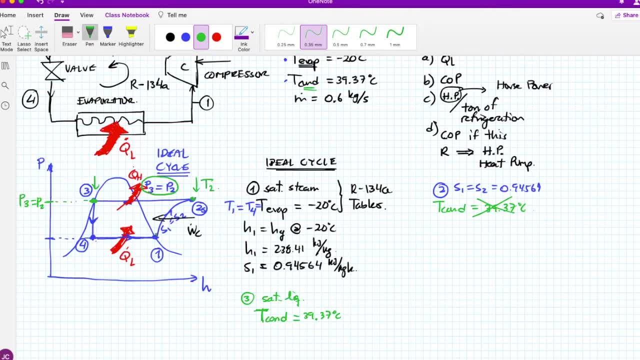 Therefore, you can assume if it's the same pressure, it should be the same temperature. It's called saturation temperature, but not here, just because of looking at this diagram. So the only thing that now you know that you can use. okay, so let's just go here. 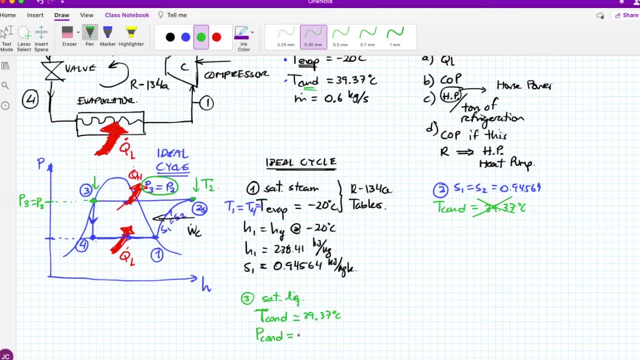 So maybe I can find here the pressure for the condenser, because if I know the saturated liquid, that it's in saturated liquid conditions and I know the temperature at the outlet. so let me just establish this as, putting these guys, T3,. 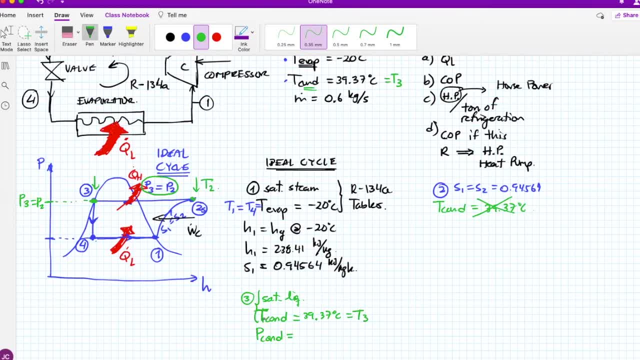 okay, at the outlet of the condenser. Therefore, you can actually find the pressure at the condenser. If you go to your table, you'll find out that this guy is located right at one megapascal of the pressure of the condenser. 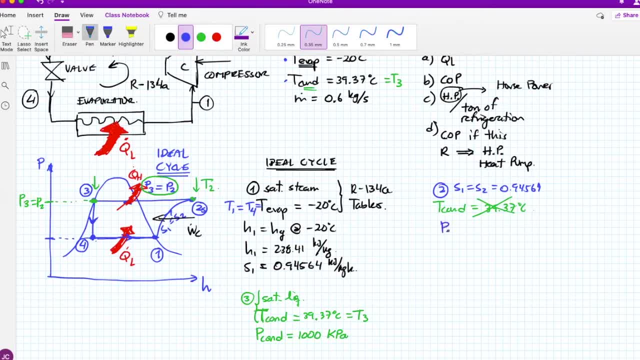 Therefore, now, what I can establish at two is that: okay, so P2 equals to P3, this is for real. okay, This is actually something that I can know. I know that the pressure is the same. I wasn't sure about the temperature. 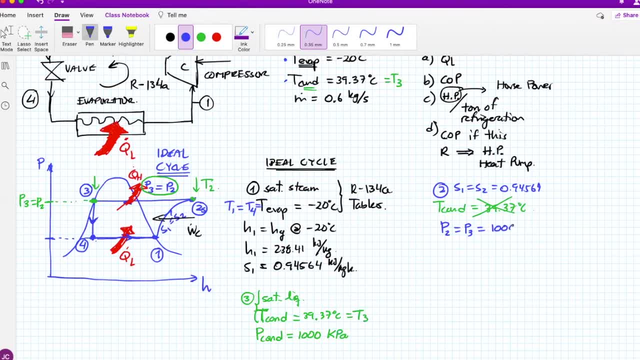 but I was sure about the pressure. So in this case, 1,000 kilopascals, And now, with these two guys, you will be able to get the pressure. I'm sorry, everything you need at two. Let me just finish. three, okay. 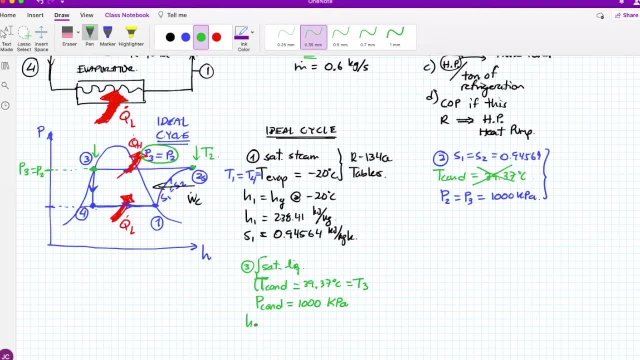 So I'm going to finish three And with these two guys, I'm able to find H3. equals to HF at 1,000 kilopascals, if you like, or maybe you would like HF at 39.37 degrees Celsius, and this is the same thing, okay. 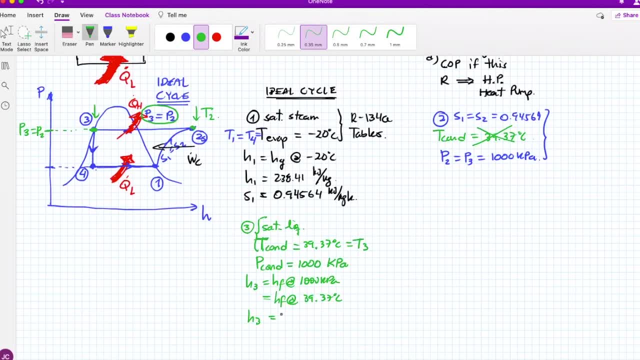 So H3 is equal to 107.32 kilojoules per kilogram. okay, So you have found yourself the enthalpy. Let's go back to two and for two. now you can actually solve it because you have two data here. 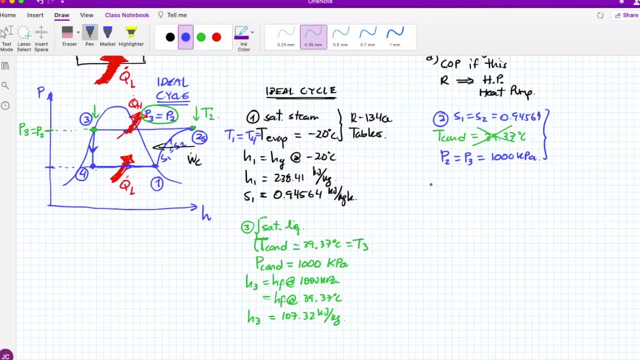 You have the entropy and you have the pressure. Therefore, with these two guys, you need to decide, decide. well, the problem's gonna give you this. So, at pressure two. at pressure two, which is 1,000 kilopascals. 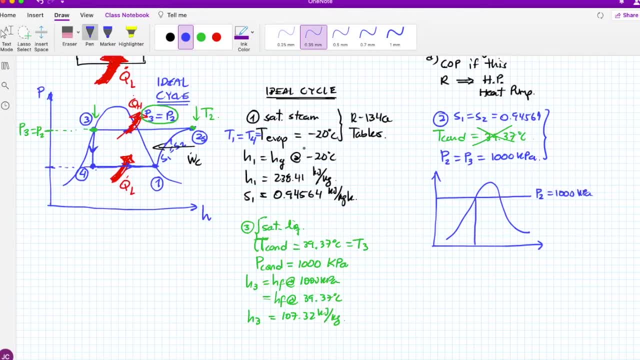 you need to figure out where the hell you are here. What do you mean? Maybe you are superheated, right, you're superheated, okay, but you can prove that. you can actually prove that you are in superheated. how so well you go to sf, the saturated liquid, the entropy of saturated liquid at this pressure. 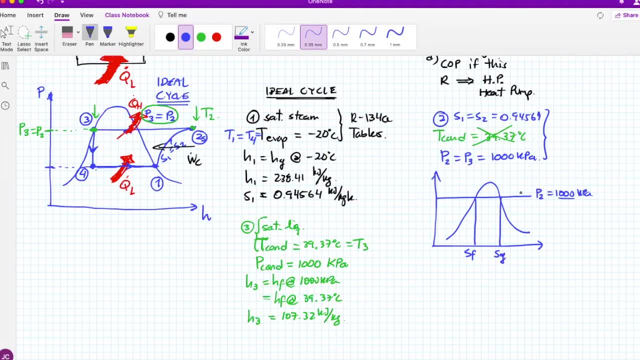 the saturated steam at this pressure and you will find out that this, that this guy is actually lying here in superheated, as we assumed. okay, so then you go to superheated. how you go to superheated, you will go to your table of superheated refrigerant. remember, this is not h2o and at p2. 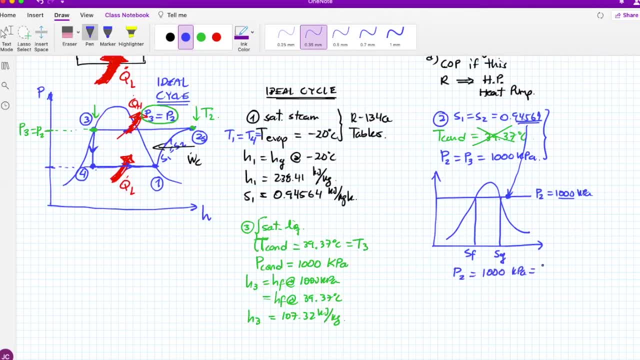 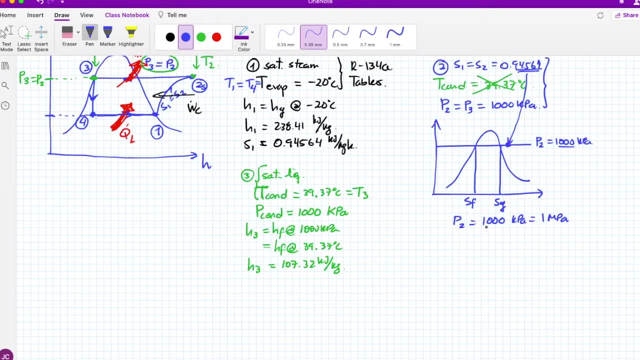 equals to a thousand kilopascals, or whether it says one megapascals, you will find out. you will find out something. you will find out that, um, there's this tablet of pressure and the other information that you have is the entropy, and you will find that you have 0.9179. 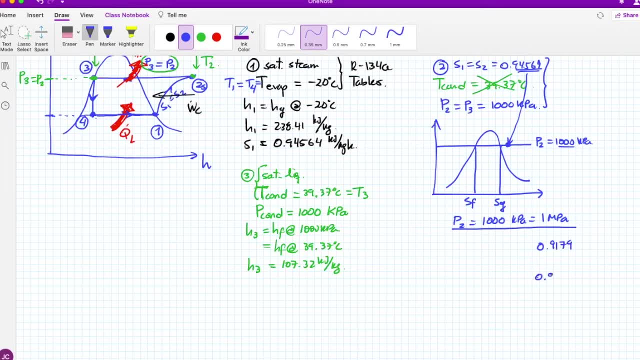 and that you have 0.95 in your tables. okay, so i'm writing what i have in the tables- 0.95, and here, here, but you don't have this fella. you would like to see this fella in the table, but you don't have it. 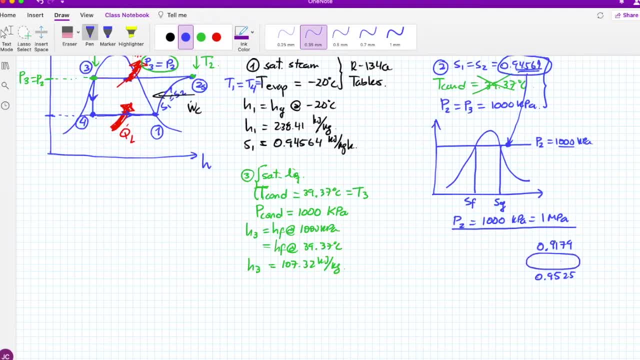 therefore, your actual value is lying here in the middle. okay, you, this is for the column for the entropies, but you also have a column for enthalpies. so for this one you will find out that you have two, i'm sorry, two. two, one point seventy one, and you have two eighty-two point seventy four. okay, so this. 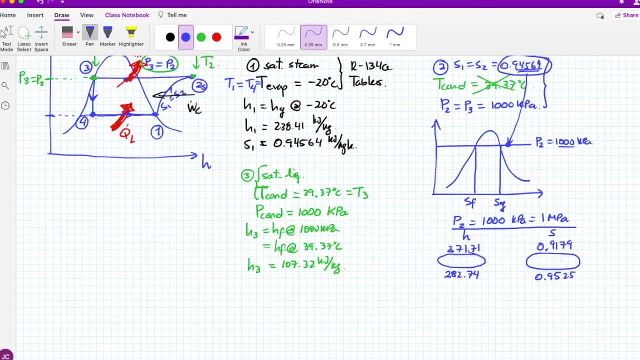 is the value that you're looking for. this is your h two, h two that you're looking for. okay, so you will place here point ninety four, five, six, four and you will interpolate. let me just put the interpolation formula. so you cannot. so you don't waste time doing the uh. 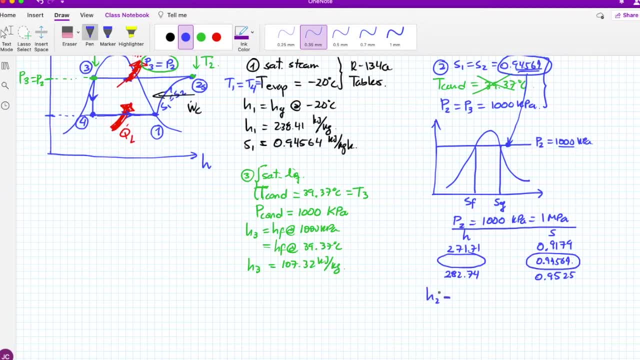 the straight line. okay, because interpolation is actually doing a straight line. so h two minus two, 271.71, and divided by 282.74 minus 271.71, equals to 0.94564 minus 0.9179, and everything's going to be divided by 0.9525. okay, minus 0.9179. okay, so good. now with this, h2 is actually 280, 280.553. 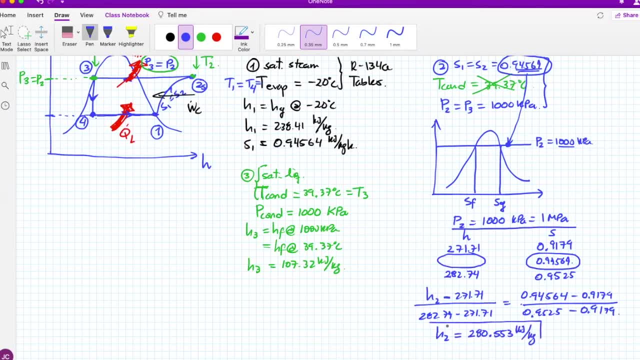 kilojoules per kilogram. okay, so it just uh, you know, it's just uh. oh, my god, i need to do this interpolation, but it's not difficult. it's maybe more bothersome, but it's not difficult. so h2, you already have it. you have h3, we're just missing 4-4. okay, so 4-4. this is really simple. 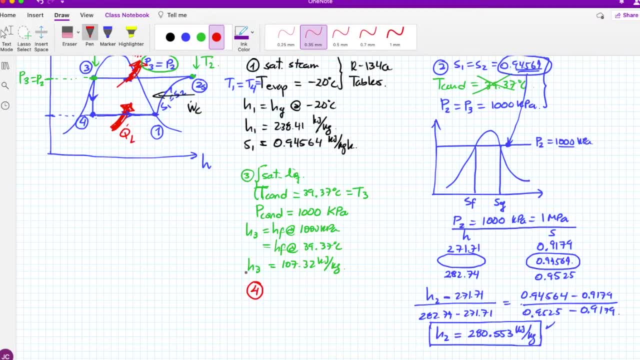 i have a bulb in the middle of 3 and 4. therefore h3 equals to h4. how do you know that? because it's a bulb and bulb the um, these, these bulbs, they do these things isentopically okay most of the time. so in that sense, well, h4. 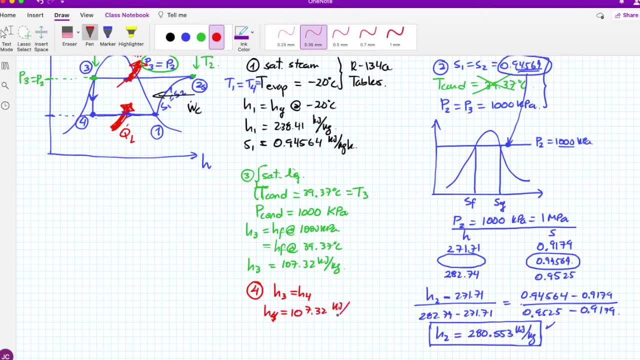 you. let me just put: h4 is 17.32 kilojoules per kilo. okay, so everything that i have placed here is just steam tables, refrigerant steam tables. you should be able to get the enthalpies that. that is the thing that will help you out to get all this stuff. okay, so i'm gonna do one more thing. 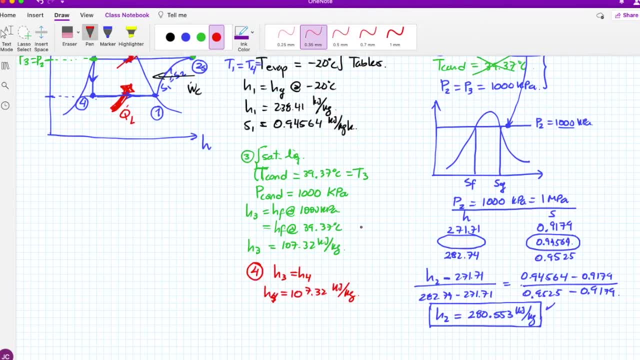 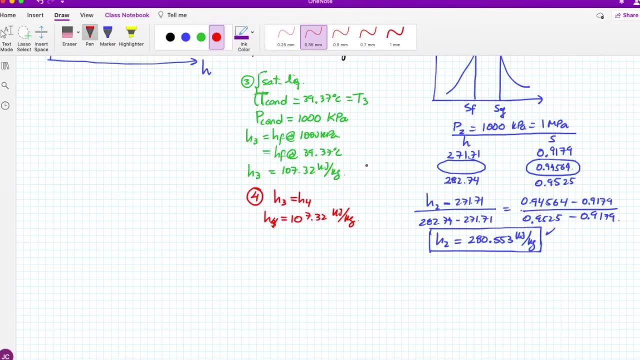 regarding steam tables. that is not. they are not asking to do this in the problem. nonetheless, i could ask you to do this in, uh, you know, in a test or something, or they could ask you to to to get something. okay, because this thing was too simple, because this was okay, so now i'm 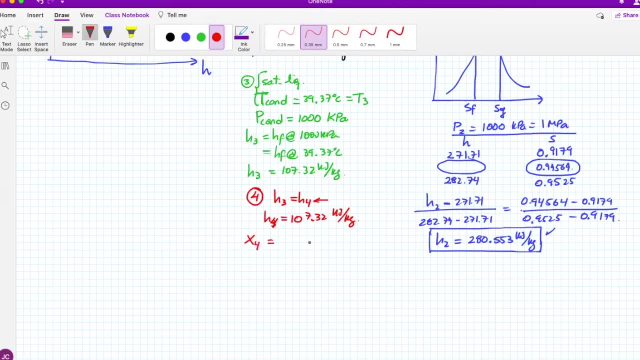 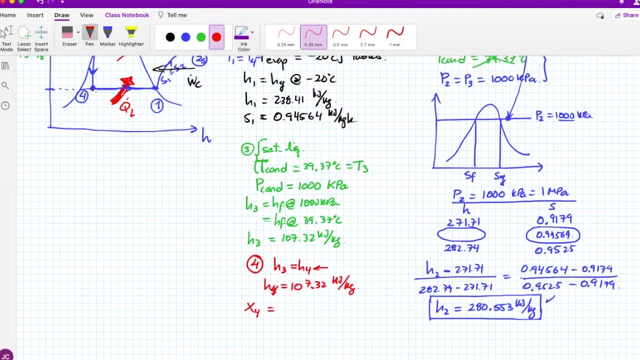 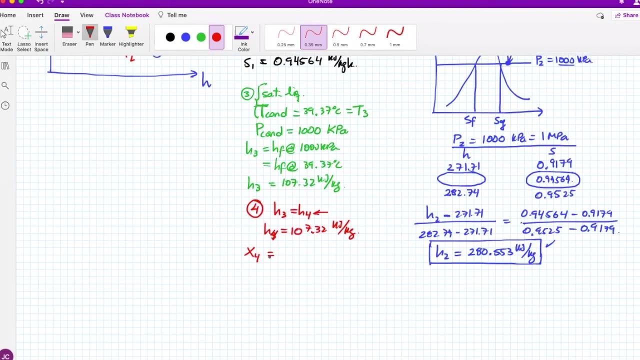 gonna, i'm gonna tell you how to get the quality, the quality of 0.4, which is this point here. so, according to this diagram, this 0.4 should be mixture right, should be right in the mixture. therefore, i'm gonna get myself the quality just to okay, just as a as a funny uh side of this, uh, of this whole story. okay, 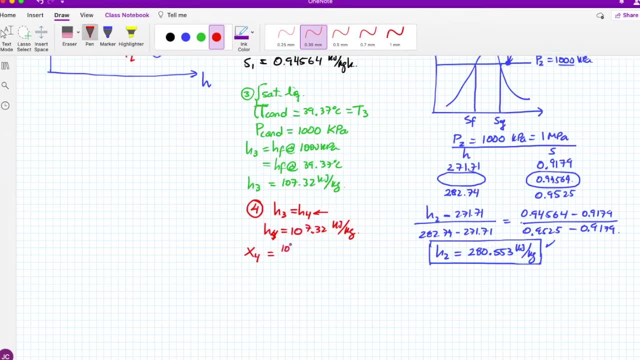 um. so, therefore, i'm gonna, i'm gonna put it: one, 7.32, okay, minus minus 25.49, divided by two hundred and twelve point ninety one, okay, how the hell did you get to this place? well, maybe you detect that. this one, right, this guy, it's actually so. you know what i have put here. this is hf at the. 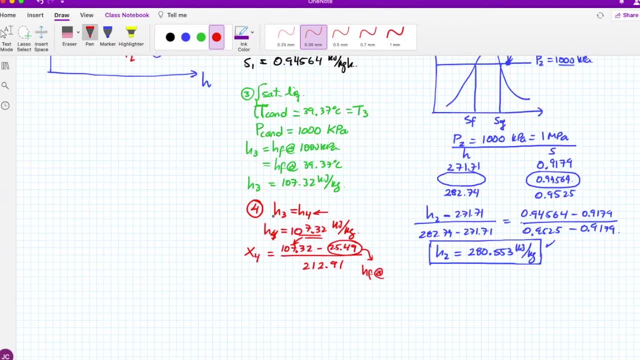 conditions of four, which are the conditions of four. well, okay, so i can put them here, if you want, at temperature of the evaporator: oh yeah, i have that. yeah, are at minus 20 degrees celsius, and this guy that you see here should be hfg at minus 20 degrees celsius. how do you know that? well, 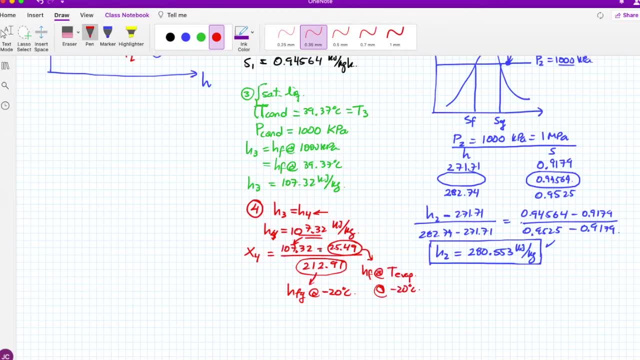 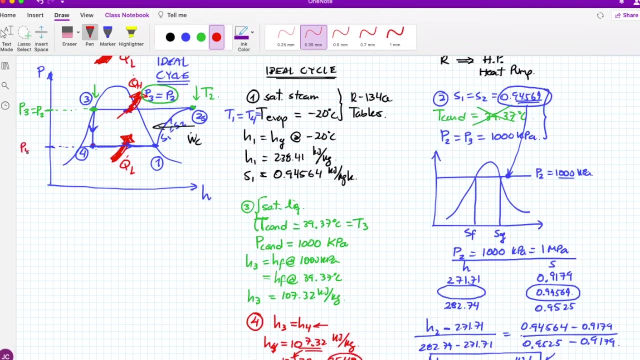 i know that i have minus 20 degrees celsius or maybe you can. you want to use the pressure? you can also use the pressure, the low pressure here, oh, but i don't have it, but you can get it right. we, we didn't use it, but you can actually get it. this one before was to. p1 should be saturation. 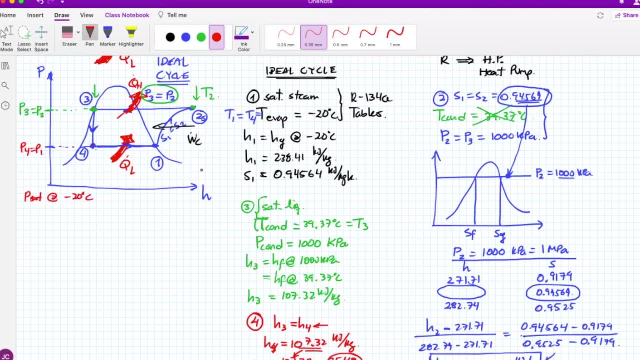 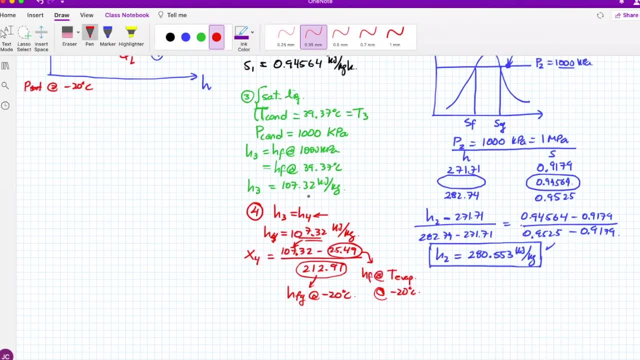 pressure at the conditions of temperature of the evaporator, so it shouldn't be that hard to get it okay. well, okay, um, remember, the enthalpy is the same one, but not the pressure. p3 is not equal to p4. okay, so that's how i got this quality. therefore, x4. x4 equals to 0.384. 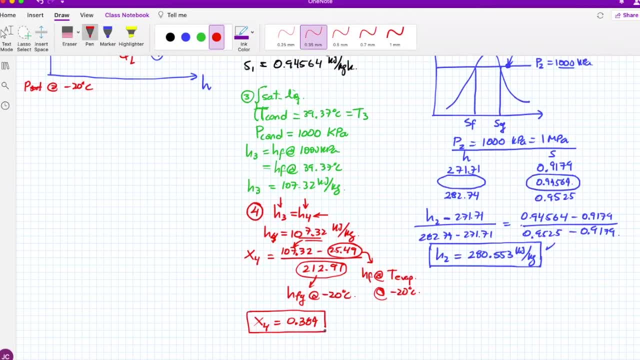 okay, so you are actually closer to the saturated liquid than to the saturated steam. nonetheless, you can have this stuff, and when you go to refrigeration and you look for the uh joule thomson coefficient, there's something that it's been used in refrigeration theory. okay, so. 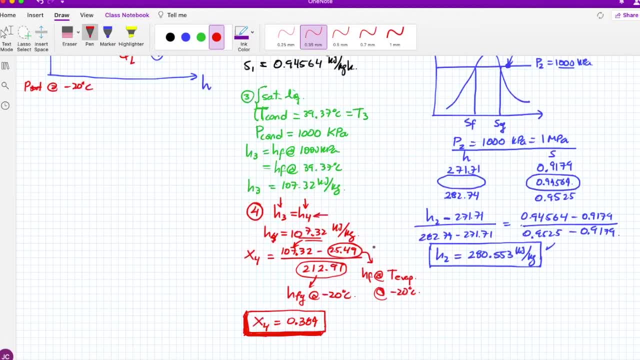 you can actually find something more about this stuff. i'm just guiding you through there. fine, you already have whatever you need. if you want, or you, you just put it into one of your cupboards. i'm just here to show you. i'm just taking the information out here here. okay, so you actually have a lot of 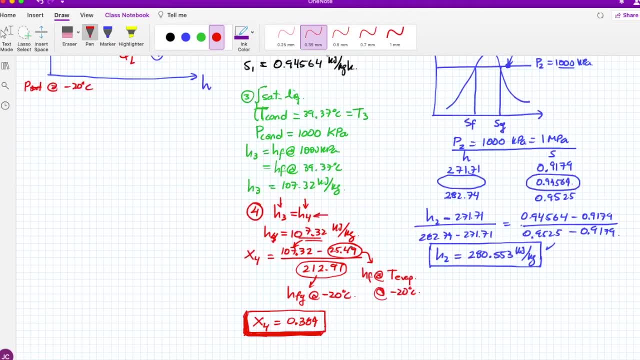 in order to get all the calculations done. Let's just try to finish the problem. So I'm gonna place it here. Maybe I can do it, Maybe I'm not going to make a mess of this. So for the, let's just see in the evaporator. 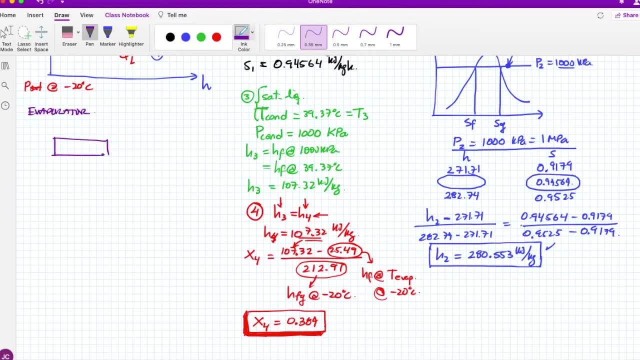 for the evaporator. you will have this, this evaporator. Here it goes for it goes out one, And remember that you have some heat going in, and this heat is called QL. okay, So QL. Therefore, therefore, let me just stick with the purple one. 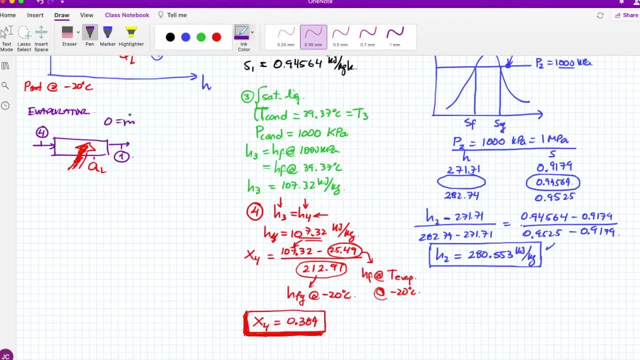 So you can do actually this: zero equals to M4H4 minus M1H1 plus QL. okay, So I'm gonna get myself explicitly a QL. So QL equals to M. remember, I'm gonna pass this guy. 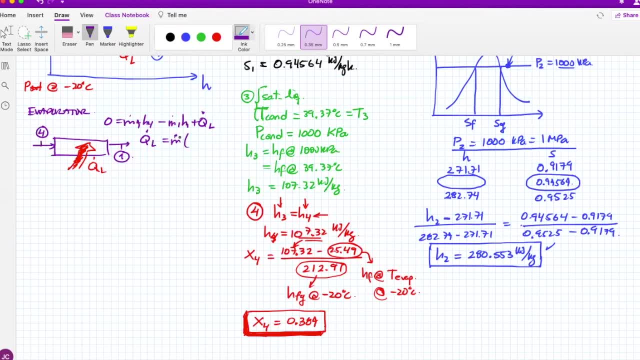 I'm gonna change the sign to everybody. So M, which is M1, or three or four or two or whatever, because it's the same one. So M equals to H1 minus H4.. This is the heat weight that I'm taking out from the food. 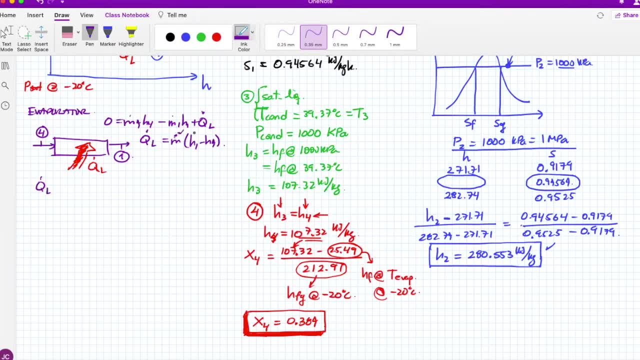 So, if you do your calculations, remember we have everything we need. okay, This from the steam tables and this was for data which is 0.6 kilograms per second. Therefore, QL is actually. what I have here is 78.654 kilowatts. 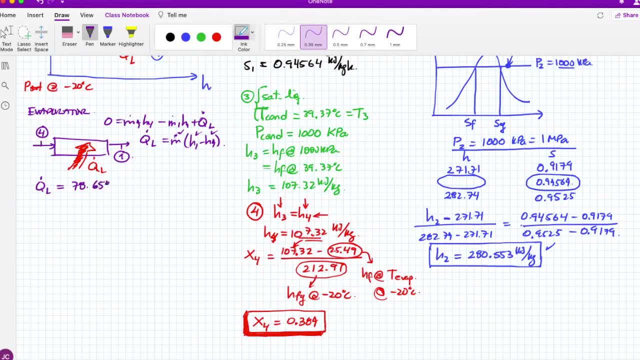 This is what I have. You can check it out and place it in the comment section. Okay, so, QL, it is like this, And what I'm going to do right now is I'm gonna change it. I'm also gonna express this in HP horsepower. 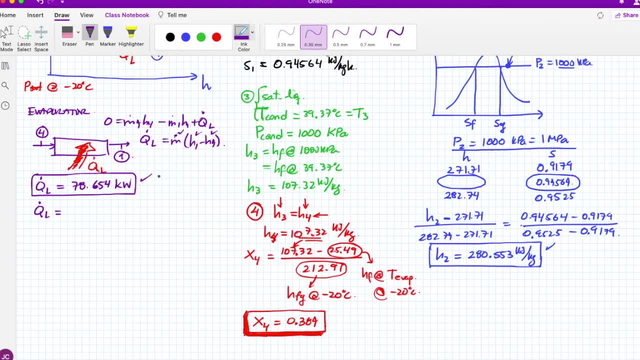 So by doing that, if you remember. so what I have here is that one HP equals to 0.746.. This is what I remember. it is okay, So maybe it could change, but do not crucify me, okay, So I'm thinking I have. 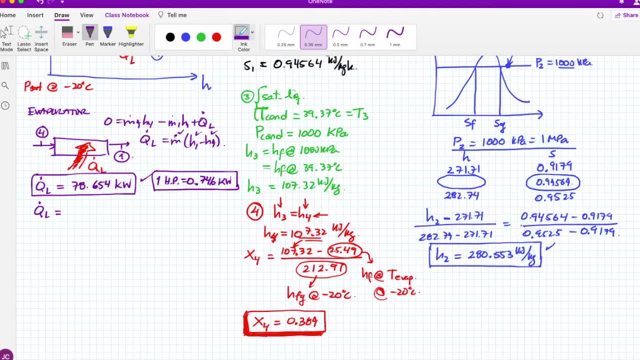 I think I remember this well, but I don't know. You could tell me. So with this unit conversion, I can get to a point that I know that QL equals to. oh my God, where do I have it? Do I have it somewhere? 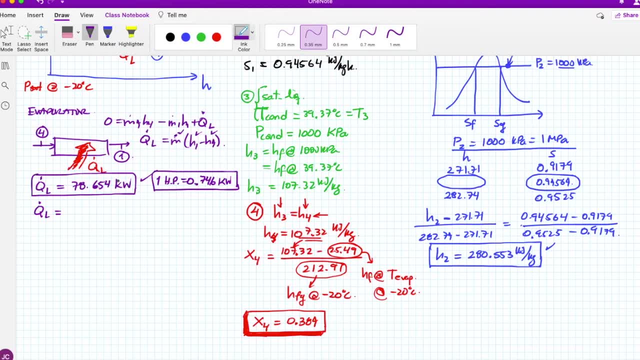 Or should I put it in some other place? Wait a little bit. Oh my God, I'm an idiot. I'm an idiot because this one QL doesn't come from any machine that produces work. okay, So sorry my bad. 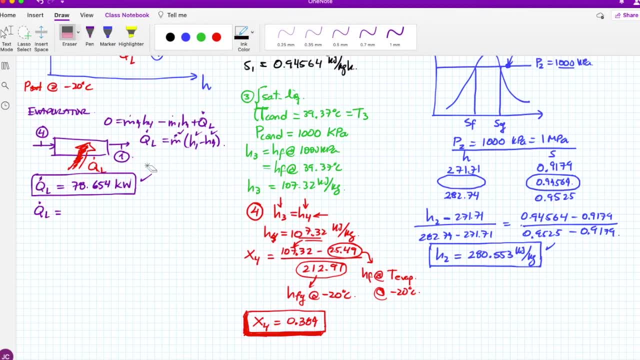 I'm gonna use that later for the compressor, but not right now. I was going all over the place. but what I can do, yeah, but what I can do is this: Oh my God, you're gonna do another mistake. Oh, hopefully not. 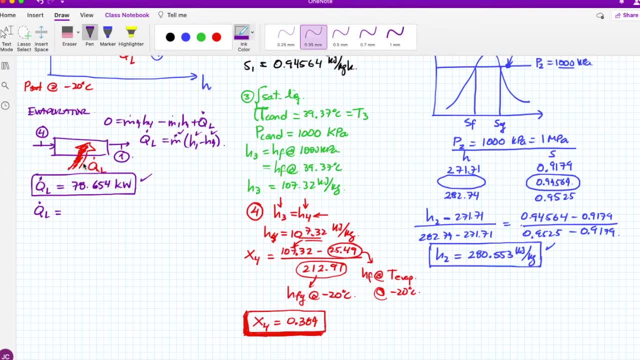 So what I'm going to do this is the heat that I just took from the food. Okay, there's a conversion. There's a conversion for this one, and I'm gonna need it in order to solve one of the things that they are asking me in the problem. 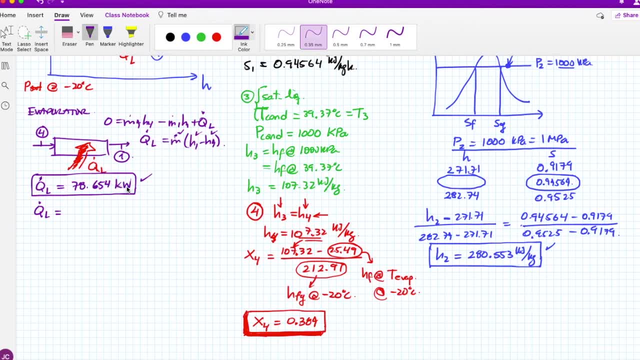 So this is the heat rate in kilowatt. but there is, specifically for the language of refrigerators, one thing that is called a refrigeration ton okay, A ton of refrigeration. that has a meaning. It's this: One ton of refrigeration, or refrigeration ton okay. 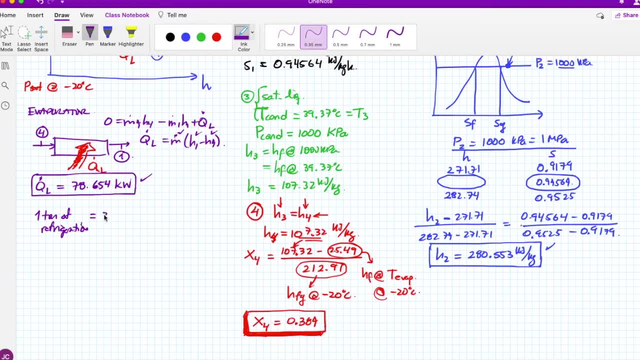 equals, if I'm not mistaken, equals to 3.5, 3.5, 16 kilowatt, And I'm gonna need it to solve one of the things that they are asking me, which is the indicator of horsepower divided by ton. 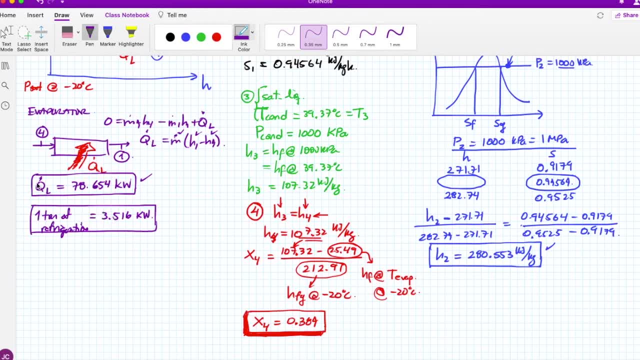 refrigeration ton: Okay. so with this I can now pass this heat rate that I got, So QL is gonna be equal to 22.37 refrigeration tons. okay, Okay, so I have that, So QL is equal to this. 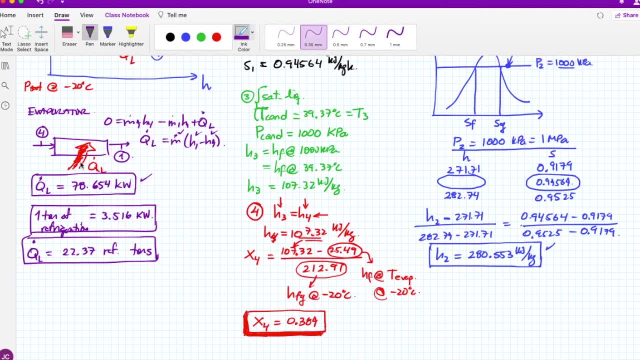 Why are you doing this? Well, if it was only about me, I could just have put this 78 and that's it. but they are asking me to put this place in some other units. These some other units are called ton of refrigeration. 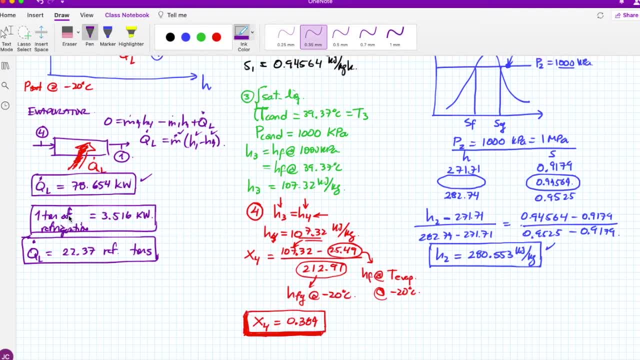 which is actually a measurement of how much heat you need to take out from a ton of water in order to produce a ton of ice. That's what a ton of refrigeration means, if I'm not mistaken. So it's actually the heat that you need to take out from one ton of water in order to produce one ton of ice. 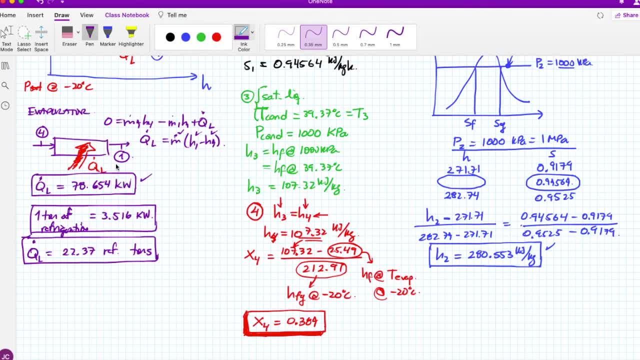 It's basically the latent heat that you're taking out of that body of 1,000 kilograms. Okay, so you already have this QL. Okay, got it. Now let's just go and see about some other stuff. I'm going to go for the compressor. 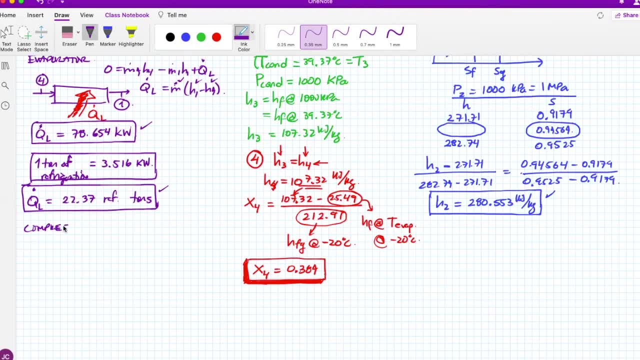 So, for the compressor, what I have here I'm going to do, I don't know if it was like this, It was this way or the other way around this trapezoid, I don't know. I actually care. 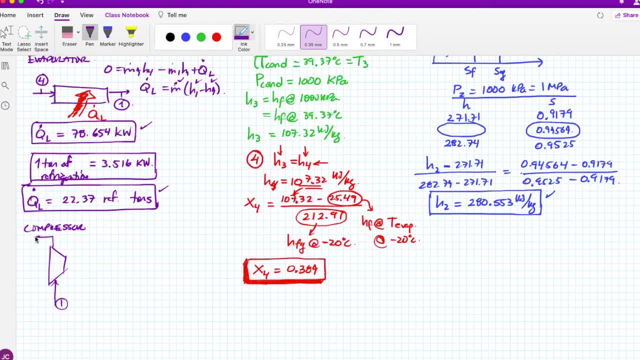 So this one is one, Okay, and this one is okay, this one is two, And I'm going to do: oh, you know you have the work going in. So this is your first law. This is M1 going in, H1 minus M2, H2 going out plus the work produced, I'm sorry, delivered to the compressor. 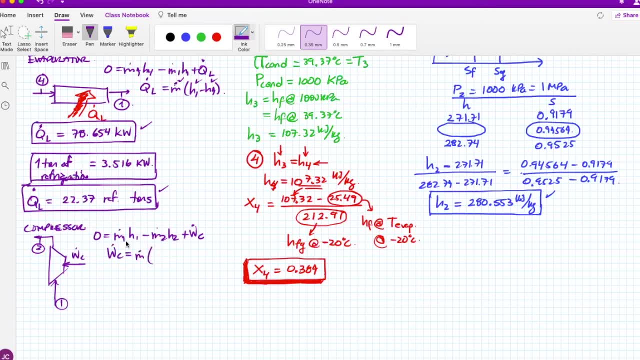 So the work is actually M, remember M1, and M2 is just M, And I'm going to pass this guy Over here. change the sign. Therefore, this is going to be H2 was negative. Now it's a positive minus H1. 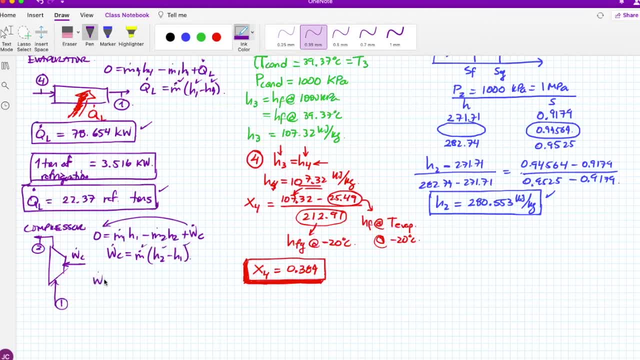 Okay, so with this you already have everything set into place, So the work produced. so again, it's not produced. It's not a turbine. The work received by the compressor is going to be 25,- 25.3 kilowatts. 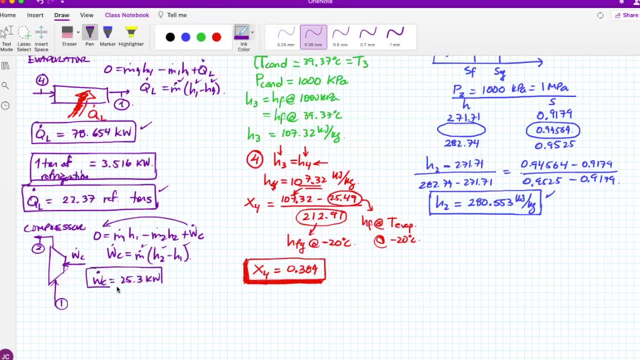 And in this case, yes, I'm going to pass it to horsepower. So again, I'm going to put again 1 HP. 1 HP, oops, equals to 0.746 kilowatt. Okay, I think you can find it as 0.75 or something. 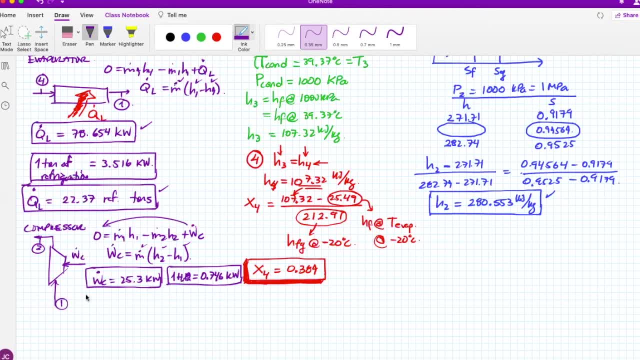 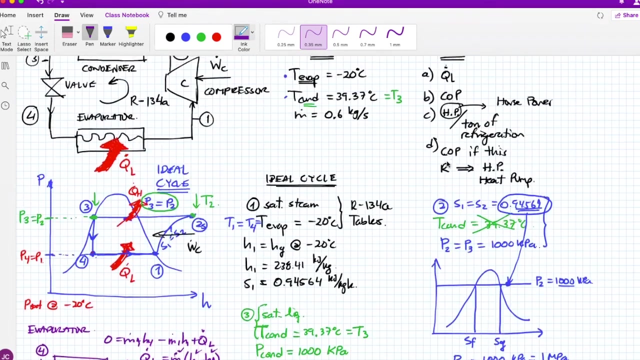 So hopefully I'm not very off from this value And therefore with this, the work received by the compressor- now I said it right, is received by the compressor- is actually 3.91 HPs. horsepowers. With this I'm going to put out of the way this thing that they're asking me this C here. 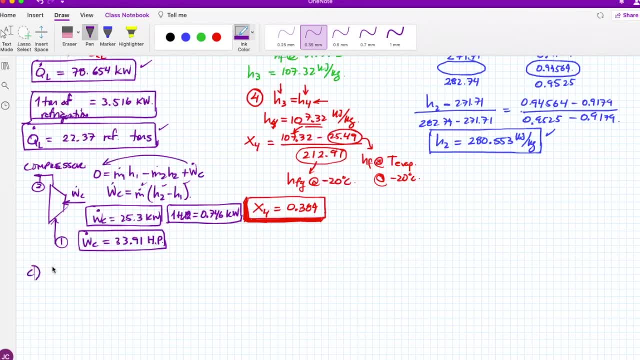 So for C? okay, so for C. I think I have everything into place. It's how much horsepower I need to deliver to the system in order to produce one ton of refrigeration. Okay, so I'm just going to do this: 33.91 HP divided by 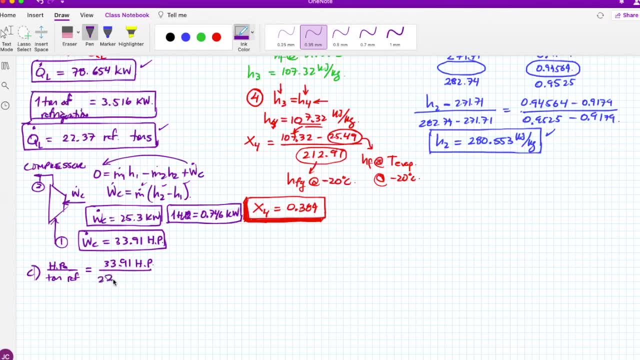 the tons of refrigeration, which was 22 point, oh my God, 22.37 refrigeration tons or tons of refrigeration, and therefore you will have yourself so again. HP divided by ton ref equals to what I have here, is 1.516.. 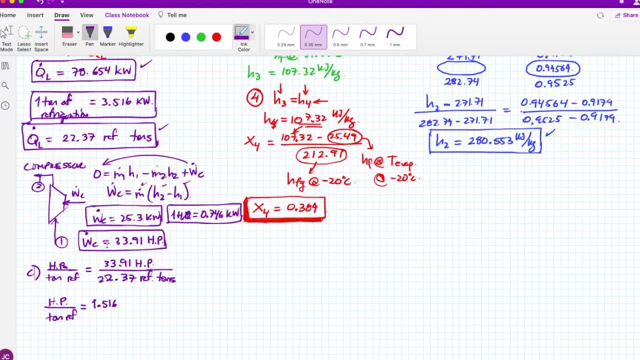 So, for every thousand kilograms of water that you want to produce into ice, you need to Deliver according to these conditions. you need to deliver to the compressor: 1.516 horsepowers. Okay, that's the. that's the idea of this indicator. 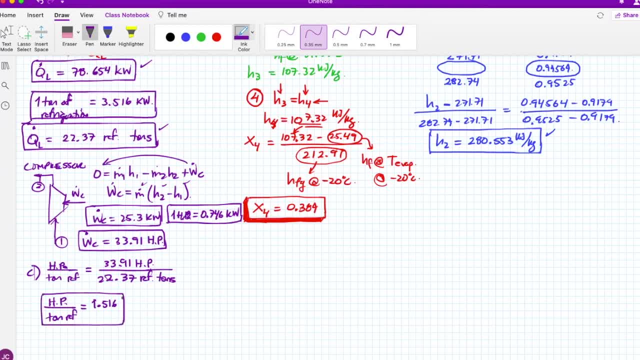 It doesn't mean that you are actually producing, you know, ice. Okay, this just means it's. it's a matter of talking about the heat rate that you are taking out of the food. Okay, it's not that you are actually producing ice. 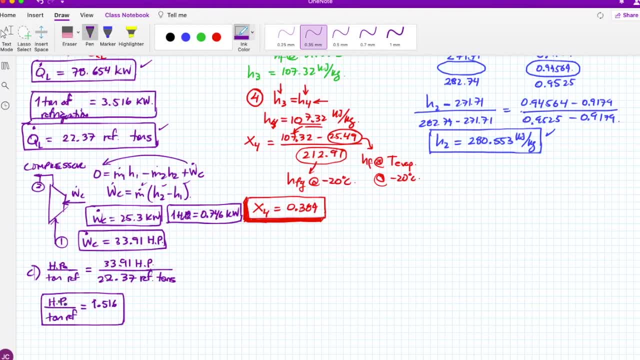 I mean you could, but it's not the idea. You can actually just Refrigerating by taking out heat, Okay. so yeah, you already have C, and but they are asking you some other things, So let's just go here. 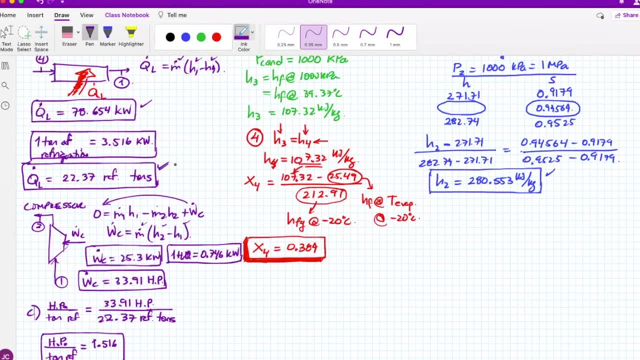 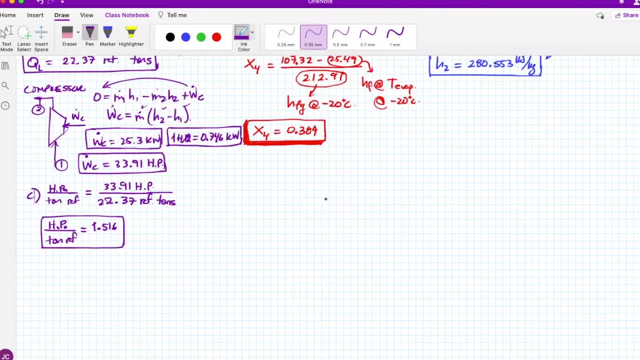 Oh, so QL. Okay, so QL got it. This one is A, or maybe this one was your favorite, So you already have A. What else they are asking me? So the cup, the cup. Okay, so the cup, it's coefficient of performance. 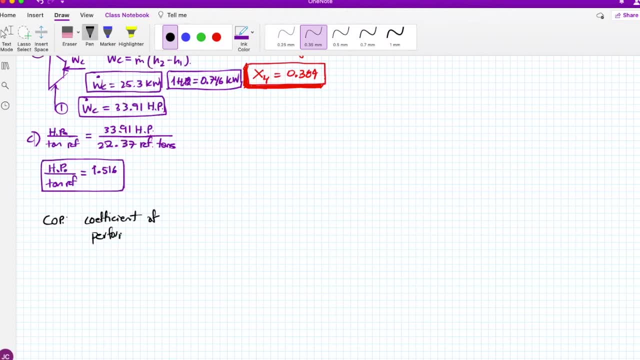 This is actually, this is actually an efficiency, Okay, the coefficient of performance. it's the efficiency for refrigerators or heat pumps that I will see later, Okay, okay. so in this case, remember, an efficiency could be, generally speaking, be defined as useful effect divided by resource. 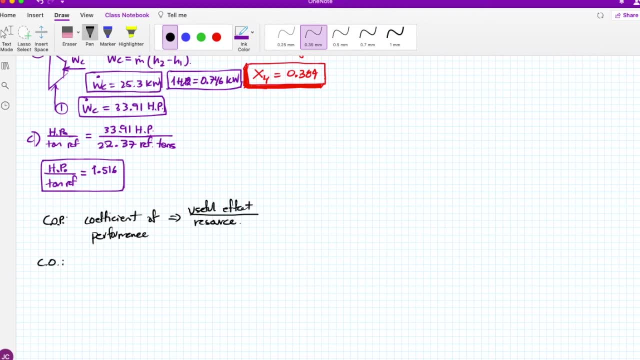 So, in this case, for your refrigerator, the useful effect maybe you catch that is the heat that you're taking out of the food. Okay, that's important, That's the. that's why you are buying a refrigerator Divided by the resource. 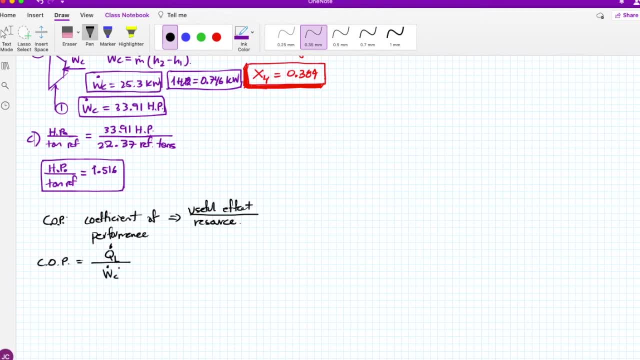 Okay, so if you don't feed your compressor, it won't happen anything. Therefore, that's the basic idea. Okay, so now you have a definition for the cup. Okay, they do not call it efficiency, in my opinion, because these values of efficiency goes farther than one. 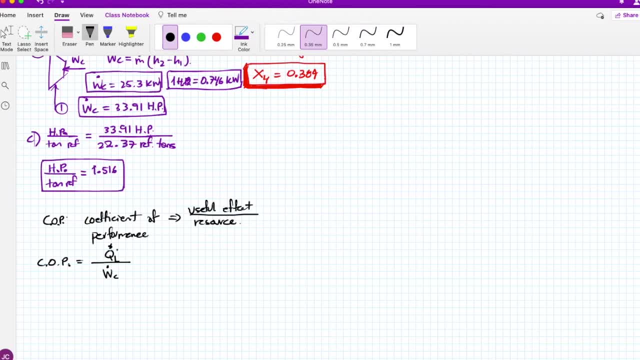 So a typical refrigerator will have, I don't know, a two cup, a three, Oh, but you mean percent. No, I mean 200% or 300% or 400%. It's a little bit off, It's a little bit confusing. but when? because when you are looking for power cycles. 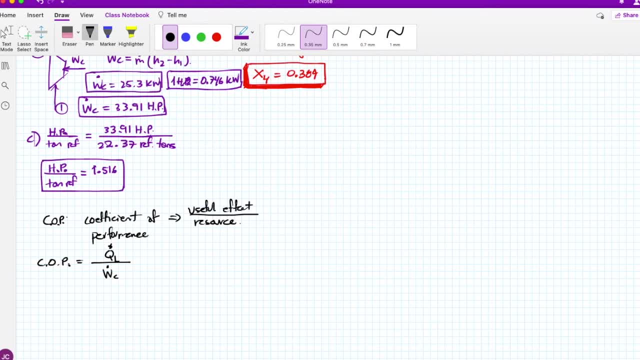 the efficiency of power cycles are going from zero to one. So when you go through refrigeration, you will find out that this also, this is an efficiency, and this guy will be farther than one. 100%. I mean a refrigerator that has a cup of one. it's a lousy refrigerator. 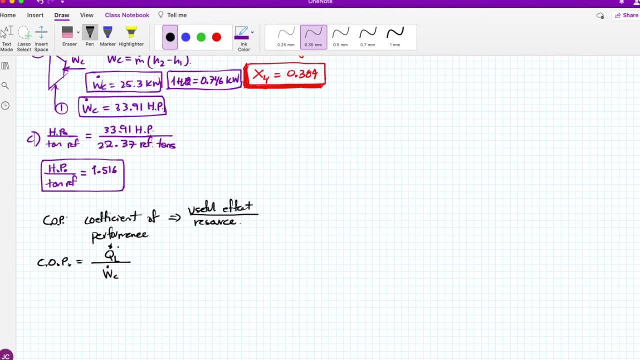 You're actually looking for I don't know three, four or something you know to say: well, this one is a really good refrigerator. Why? why it? It is farther than one, just because of the definition. you are defining some other thing. 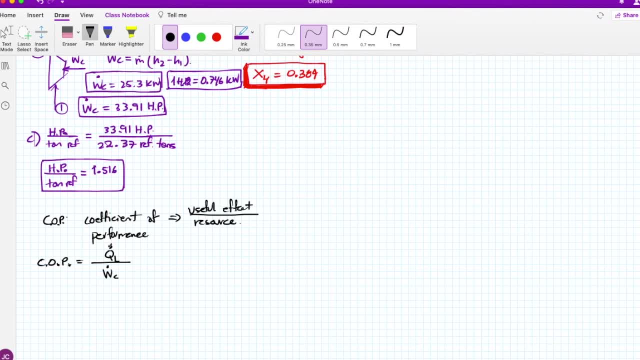 in some other way the the efficiency, And I will tell you at the end of the problem, because they are asking us something about a heat pump. So the definition of the cup for a heat pump is different than the definition of cup for our refrigerator. 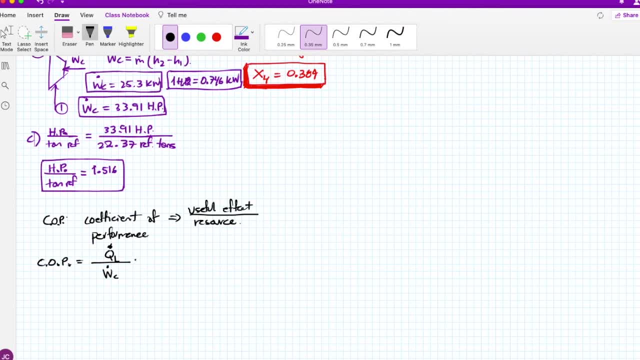 So it will change. So do not get freaked out, freaked out by the values of these efficiencies. Okay, Okay, Okay. We are not violating any physical law, It's just the way that you are defining efficiency, Okay. So, with this in mind, QL, you already have it. 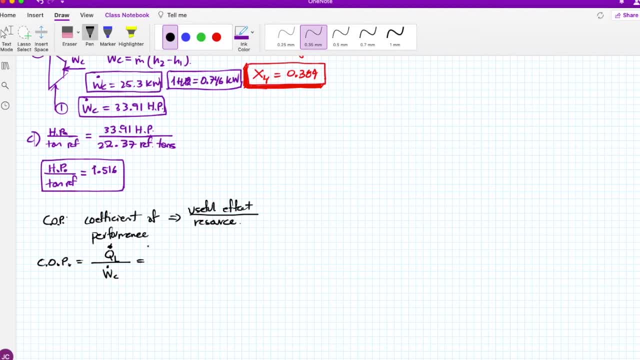 Okay. So what I'm going to put here is, um, what I'm going to put in, I'm going to put them, which is: where do I have it? Oh my God, I don't have it here. So, um, I do. 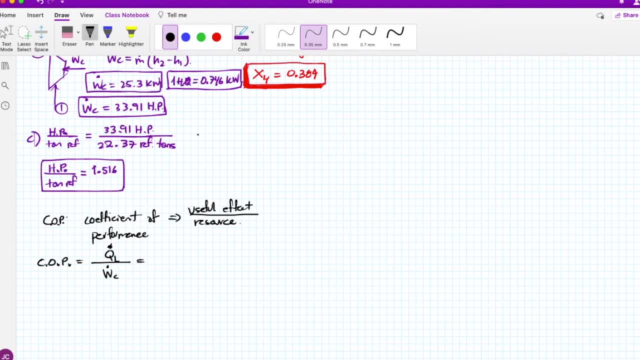 Um, I really I don't, I do not have this, Okay, So so now I have it. Uh, I didn't I said and I said, okay, I'm going to get it, Okay, Off screen of of uh, this, this video, but no, I actually just find it here. 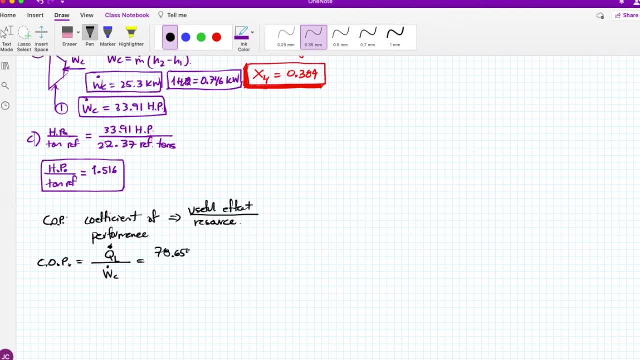 So this thing will be about 78.6, five four. this is in kilowatt, I hope, And this wise this guy is 25.3 kilowatts. Therefore, The cup will give me 3.11.. 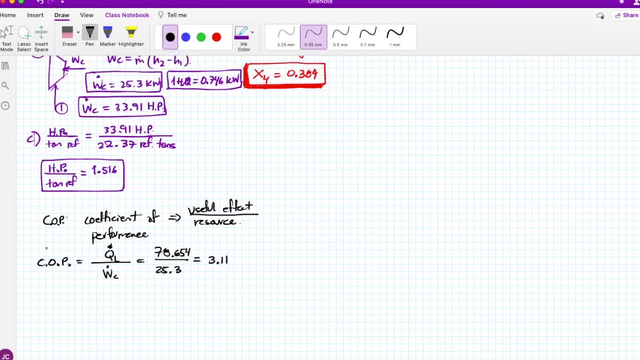 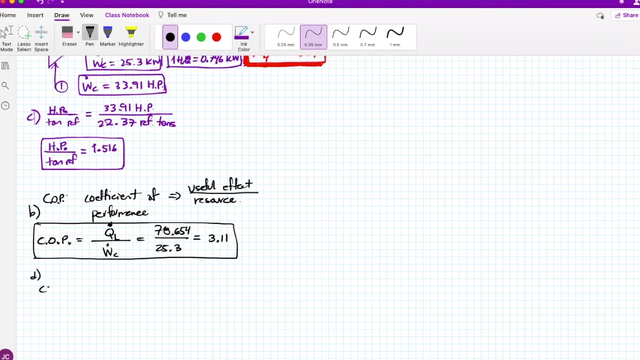 This is the cup for the refrigerator. Okay, So these guys actually what they were asking me at V. So this is B. good, Let's do one more. The one more is they are asking me. Okay, So D, let's just find this cup. 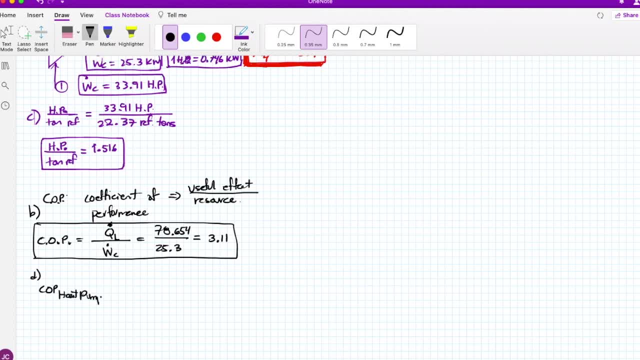 If this guy was a heat pump. so a little bit of theory. Okay, This is our Refrigerator, the refrigerator, you will play some machine. Okay, You will feed it with work for the compressor, You will take out heat from a lower reserve or temperature, which is basically. 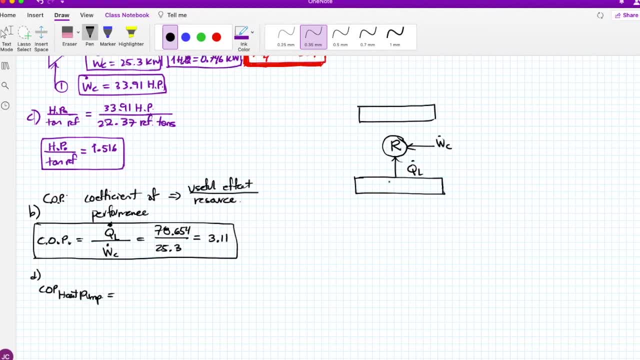 something which is um, a um, something cold. Okay, So you want to play to keep this uh reservoir cold. That's the inside of your refrigerator. Th is where you're throwing out the heat And you want to put in the condenser. 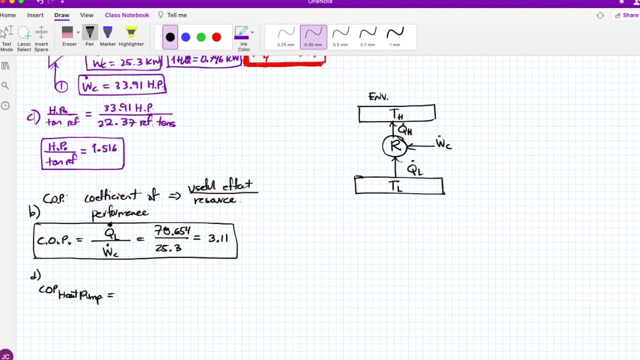 Okay, So basically, this is the environment, This is the environment And this is I don't know. this is the food. Let me just put it here. This is the food. So this is how our refrigerator can be schematically put or place in a, in a thermodynamic sense. 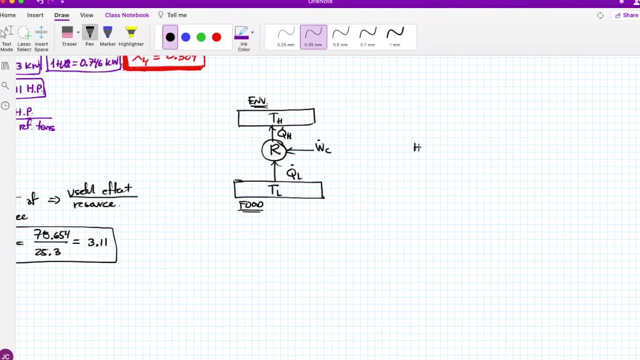 Okay, And now here comes a heat pump. a heat pump. Let me just use again HP because of heat pump, not because of horsepower. you will feed it with a work for the compressor. Okay, Okay, Okay. So you will take out heat for the. oh my God, you're going to do the same thing. 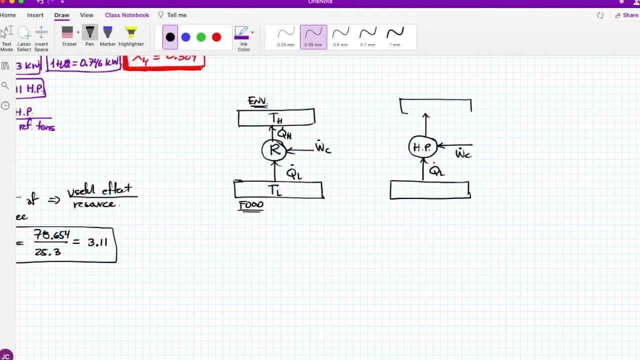 Yeah, I'm going to do, actually do the same thing here. and you will say: well, there is not a difference between a heat pump and a refrigerator. And I can tell you, yeah, there is a difference. The basic difference is that a heat pump is placed, most of the times, below a home. 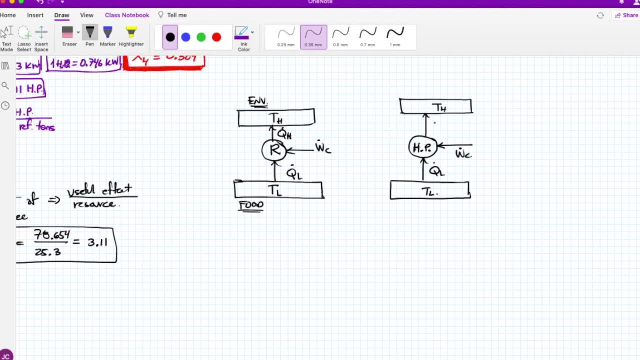 Okay, Or uh, you know a house in order to heat it. What you're actually doing with this machine is you're taking heat out of the snow, maybe, or the, or the pavement that is a little bit cold, or the ground, or the air, whatever you want to call it. 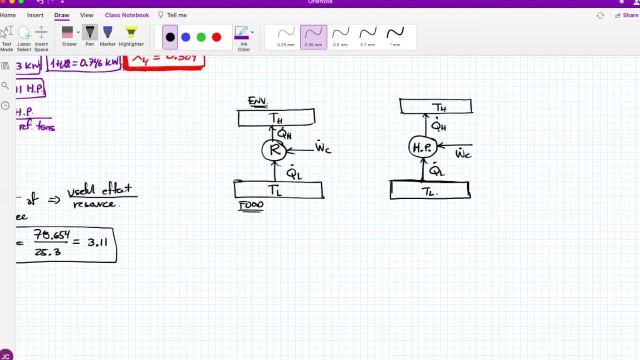 Okay That it's really cold. You're taking heat out of that and you are placing heat inside your home so that it's warm there. That's the basic idea. It's a refrigerator If you want to put a heat pump at home. 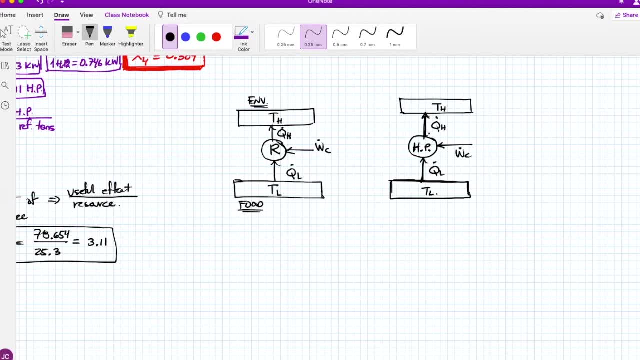 Okay, So turn around, Turn backwards your refrigerator, just place it, place um the piping that it's at the back of the refrigerator, pointing at the living room or at the, you know, at the kitchen or at your bedroom, or whatever you want to call it. 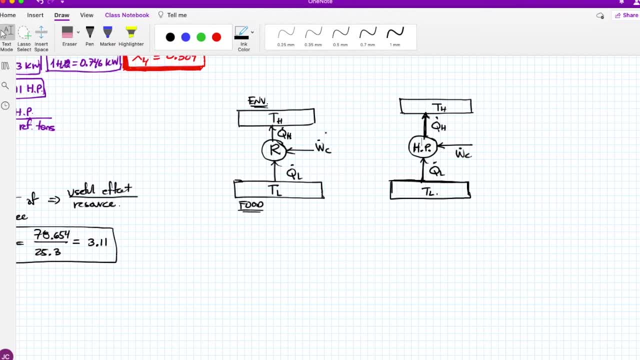 And therefore you will feel the warm. Maybe it's not very- you know very useful. That's the basic idea of a heat pump: that you can warm something or heat something by taking out heat from some other stuff. Okay, So in this sense you're not using. 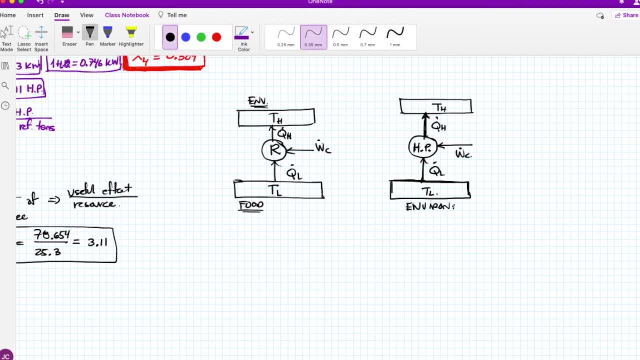 Food. You are taking heat from the environment, from from the snow or the cold round below your home, Okay, And you are placing these. this is I don't know. this is the interior or the inside or the interior of a home, of a place that you want to keep warm. 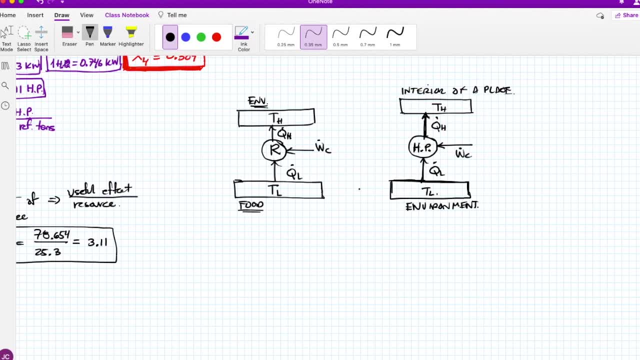 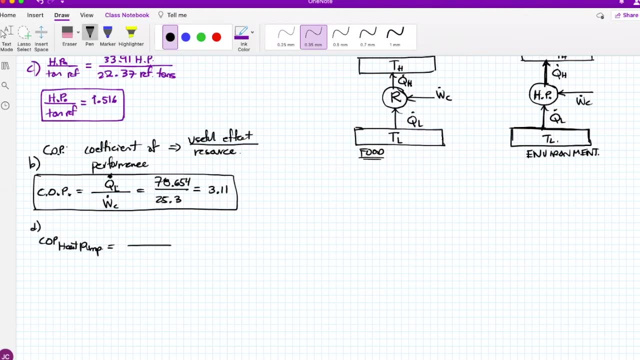 That's the basic idea of heat pump. Therefore, therefore, Okay, So I'm going to go here the cup for a heat pump. It's no longer QL divided by WC. Look at this: What is would be the useful effect. 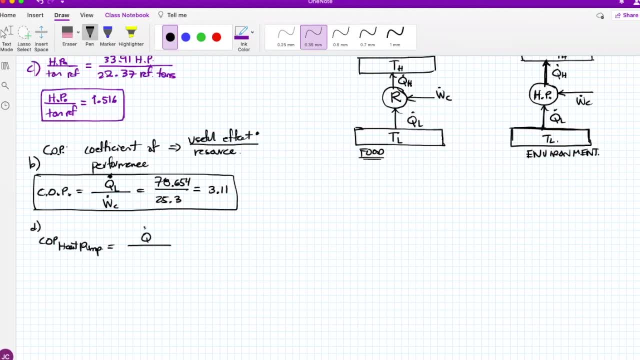 The useful effect for a heat pump is not QL, It's QH. That's the basic idea. That's what you want in a heat pump, And the reason is the same one: If you don't feed it, okay, your compressor won't move. 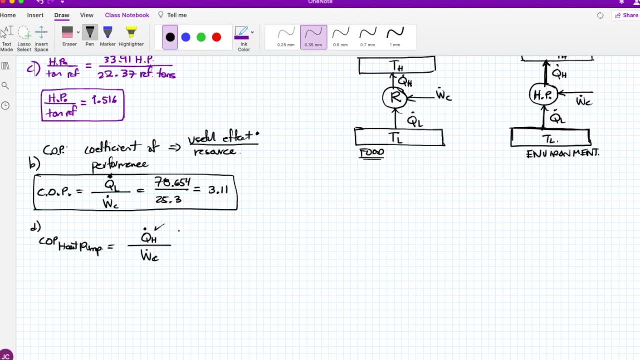 Okay. So with this idea in mind, you need to get this guy first. You don't know it. So QH is a condenser, So I'm going to rush myself here, Okay Well, why should I rush it? So here? you have to remember, this is the entrance of the condenser. 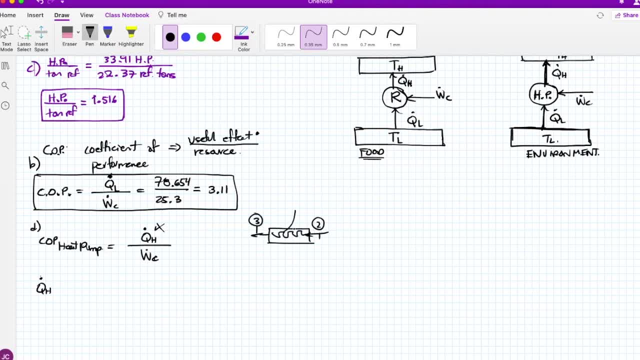 It goes this way, which is three. Okay, This is where you are taking the QL. Okay, This is the one that you're looking for- I'm sorry, QH- And therefore you're going to establish the first law.